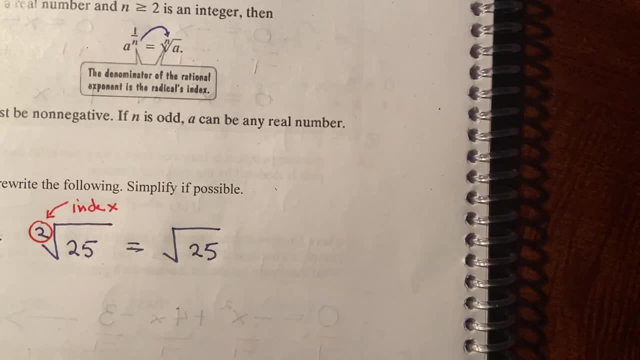 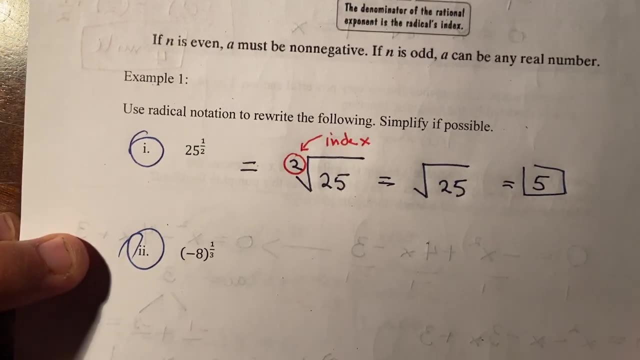 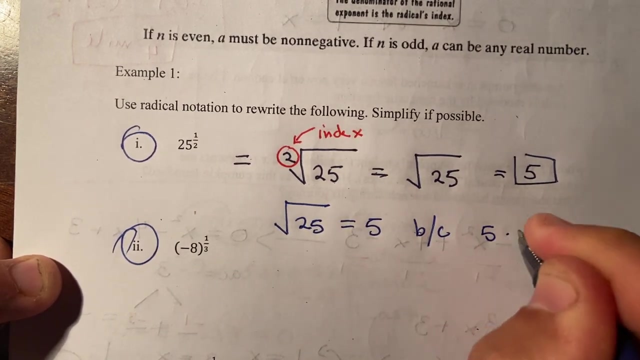 It says it's 5.. So why is that? just a quick explanation: The square root of 25 is 5, because 5 times 5 is 25.. Do the same for the other 5 turns as well. Let's try it again. 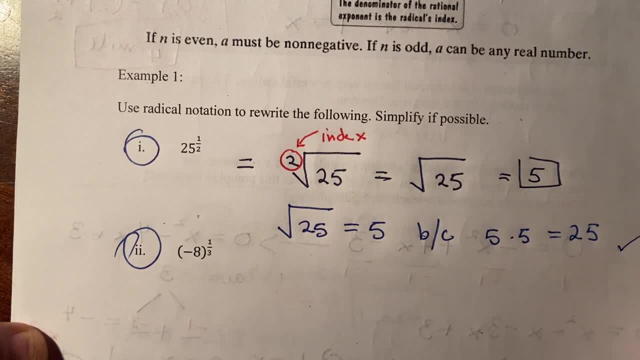 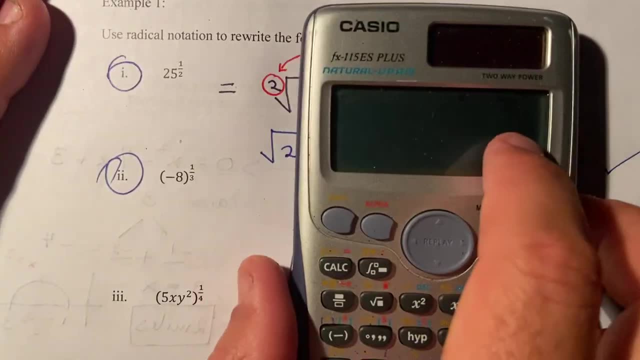 So this is square root 25, and this is the square root of 25.. So this is just a check here. All right, so the answer is 5.. You could have also just plugged this in how it was right. I could plug this in how it was. 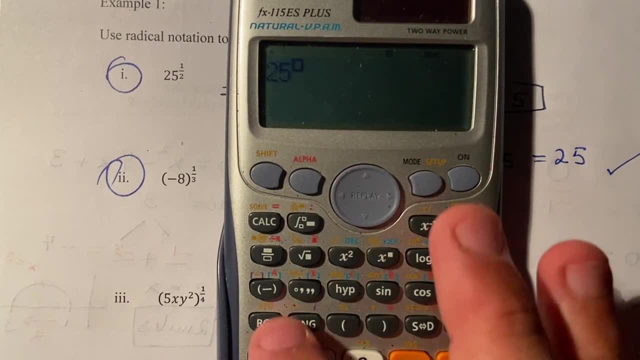 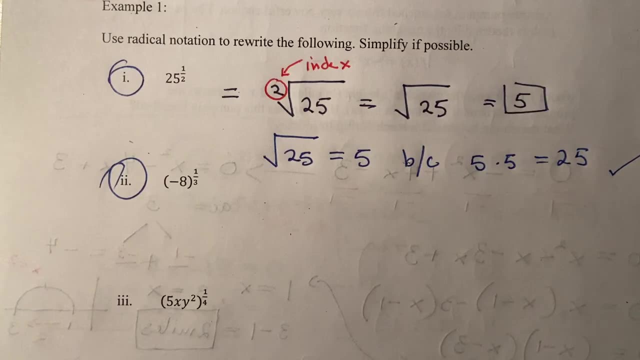 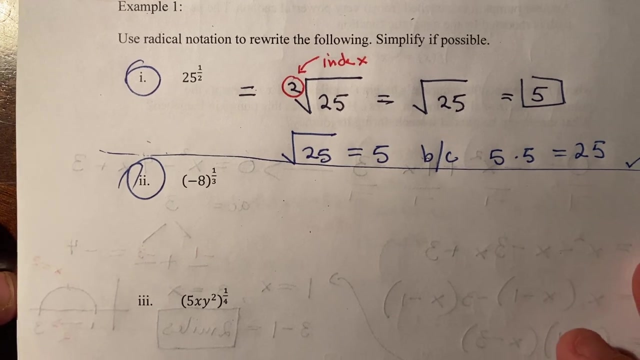 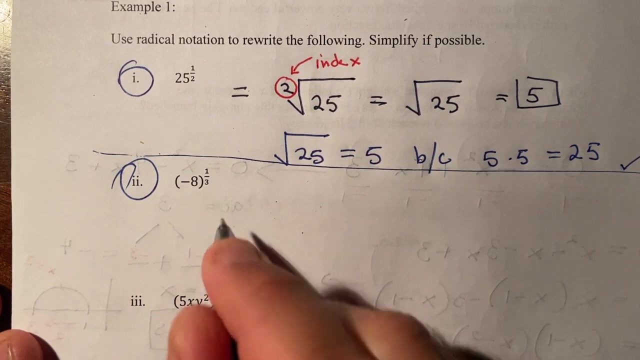 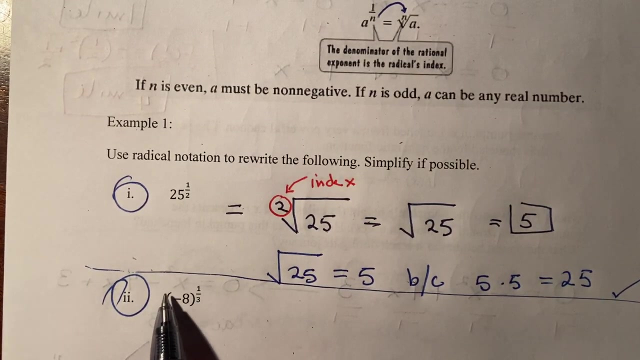 So 25 raised to the 1 half should be the same number. So what about a different type of power? Now we have negative 8 raised to the 1 third. So just to follow this up here, if we have a is now negative 8, and it's raised to the 1 third. 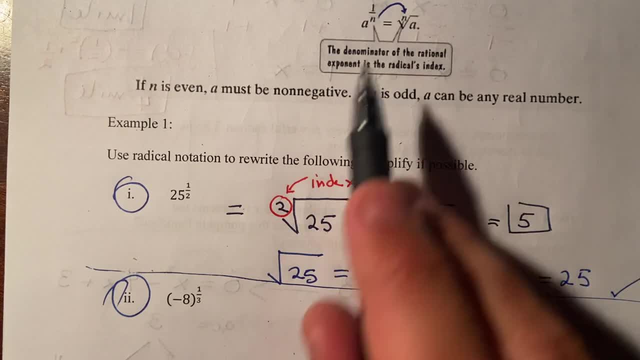 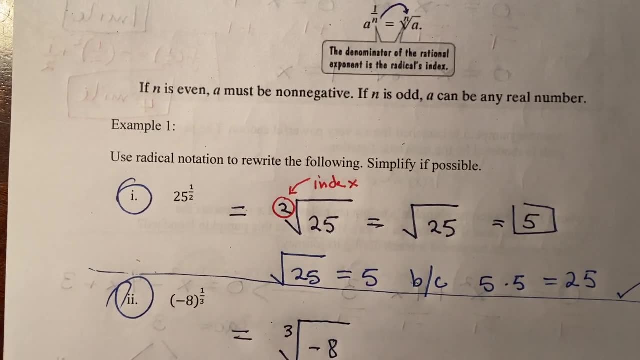 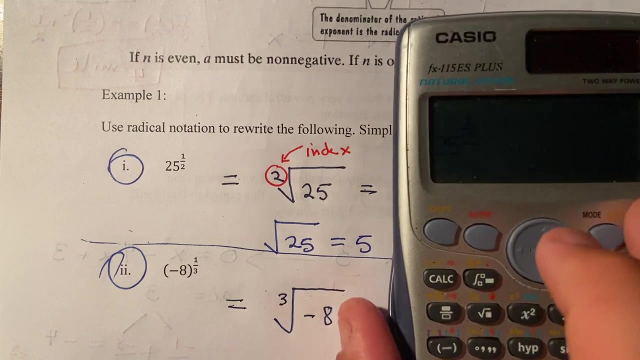 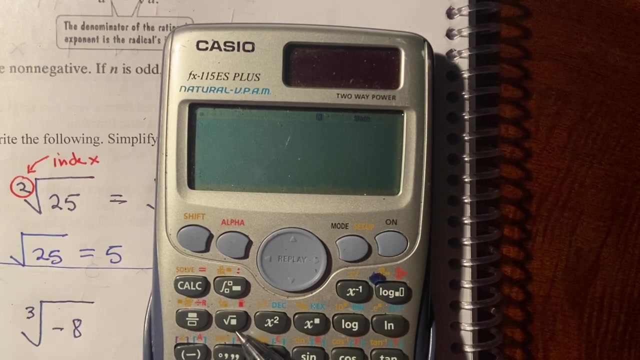 so that means that that 3 is going to become the type of the root. So this would be equal to the cube root of negative 8.. And maybe I'll type that in just to see if my calculator knows what that is. So the cube root is actually behind the square root. 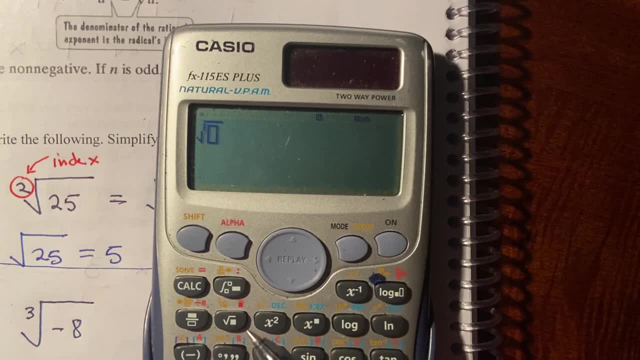 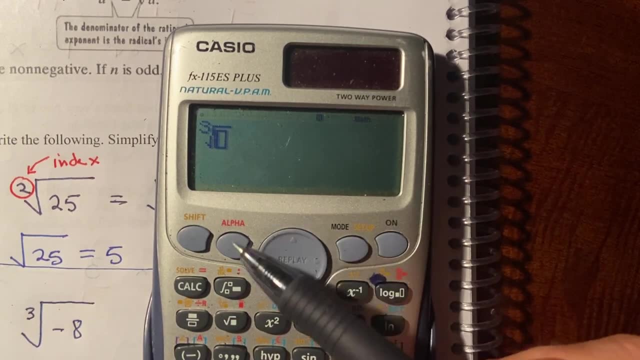 So I'll go shift and then square root. Looks like I need to press it better: Shift square root and see how cube root pops up. So that was shift, square root. Okay, So here it's a cube root and then type in a negative 8.. 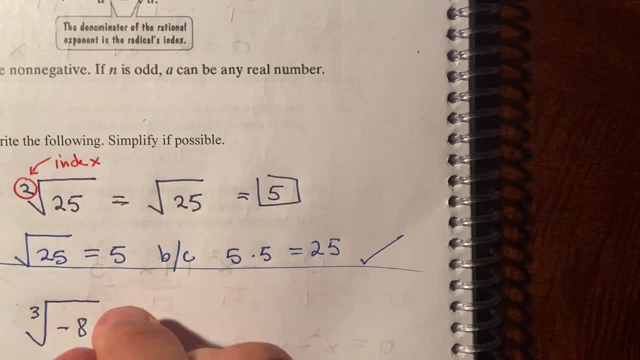 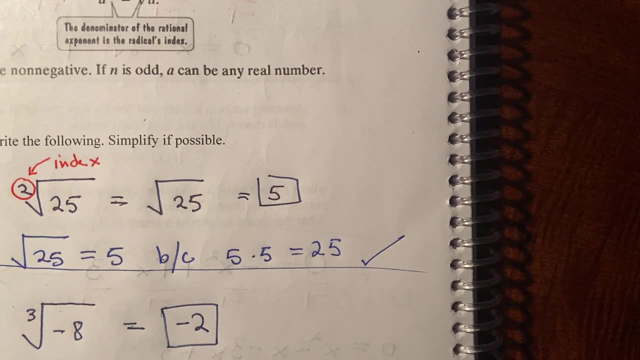 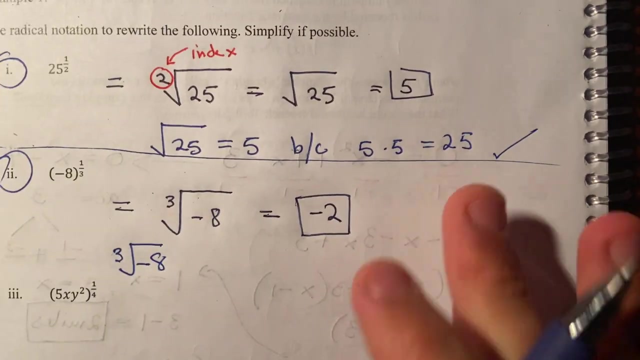 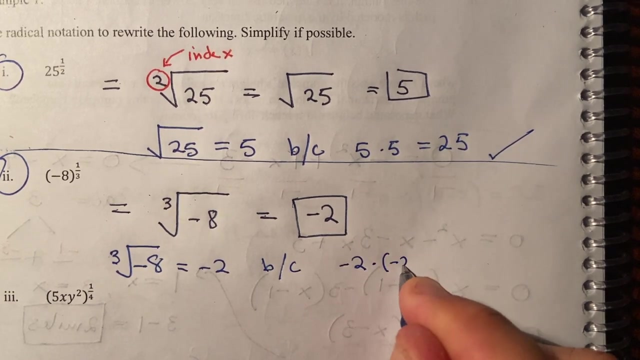 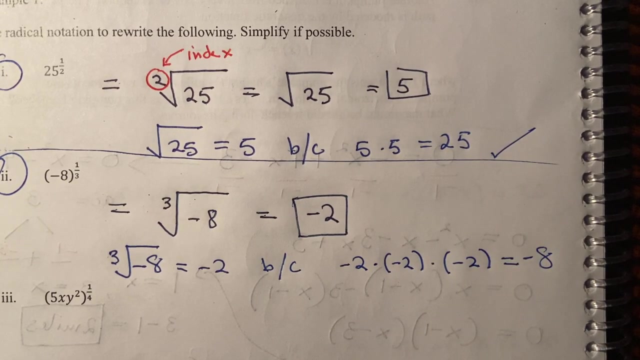 So it says negative 2.. So this is negative 2.. And this is negative 2 because Because negative 2 times Negative, 2 times negative 2 equals negative 8.. And that's what a root means, And we'll talk more about that in a little bit. 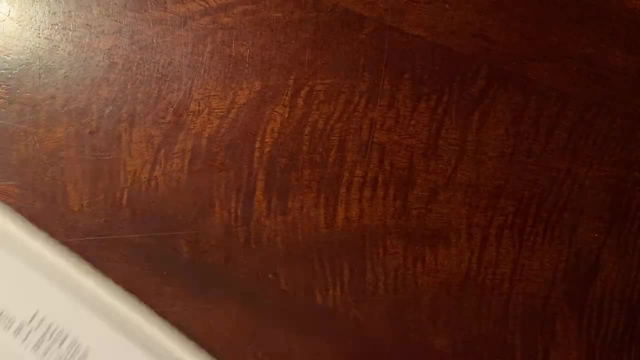 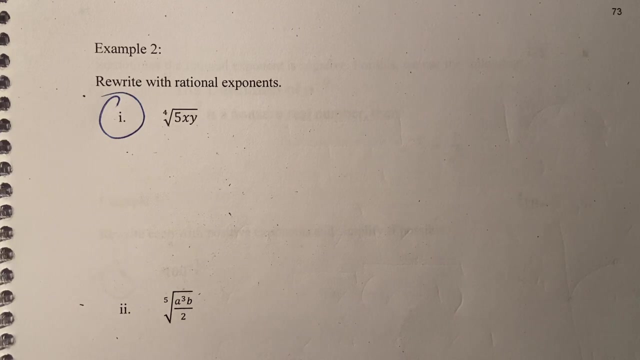 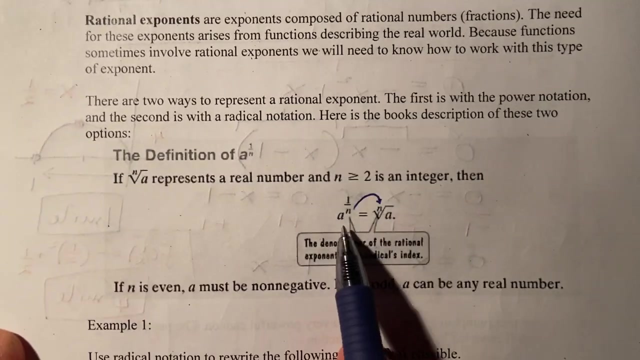 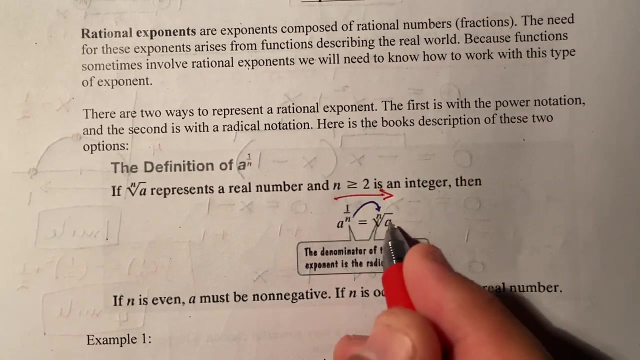 But we would have just negative 2.. So you want to be able to go either direction with that. So what we were just doing was going from left to right. So we were just going this way across the equal sign. But you can also go the other way, right? 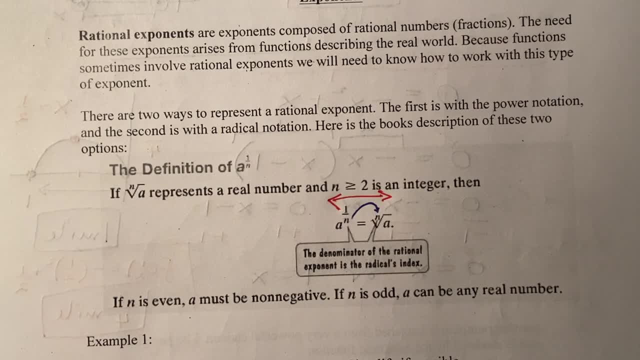 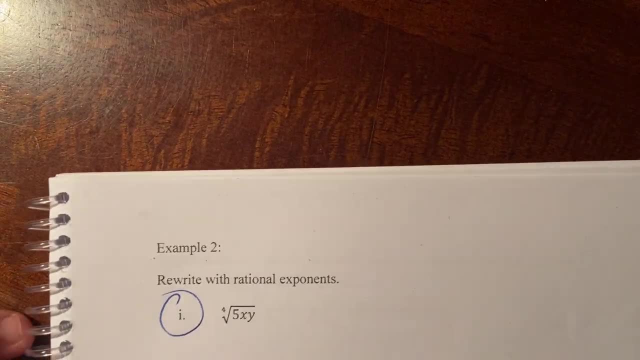 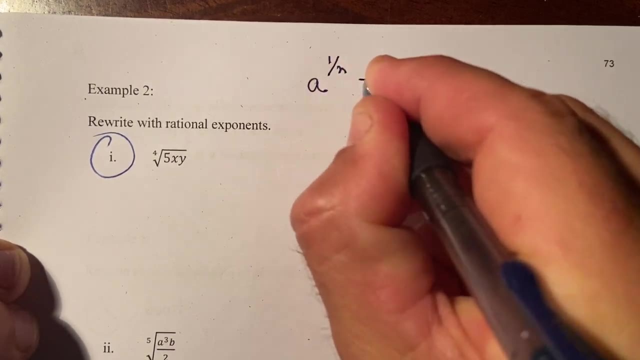 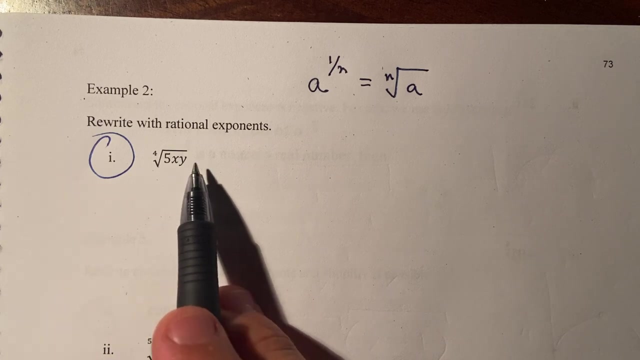 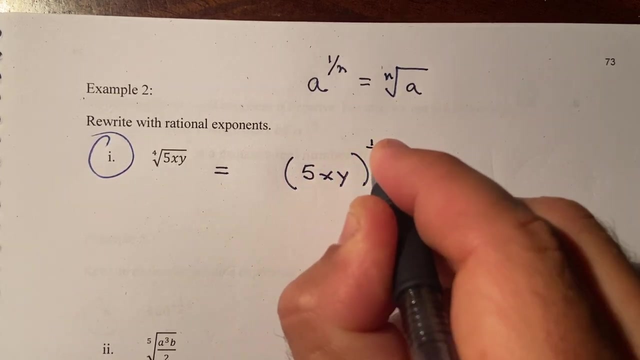 You can start here and then rewrite things as powers if you want, which sometimes is beneficial. So it said, So it said. But if you have a to the 1 over n, that's the same as the nth root of a. So if I have the fourth root of 5xy, this would be the same as 5xy all under this one-fourth power. 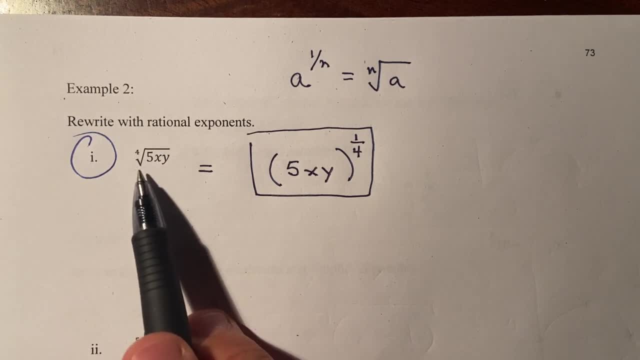 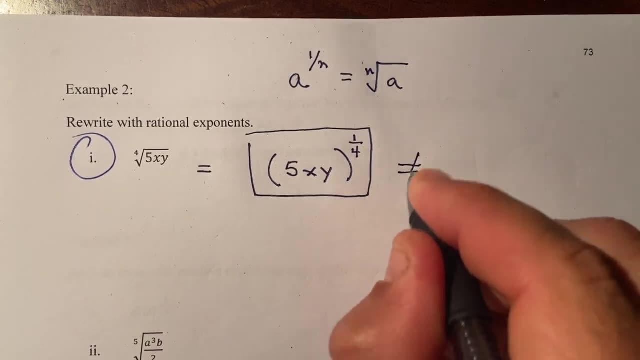 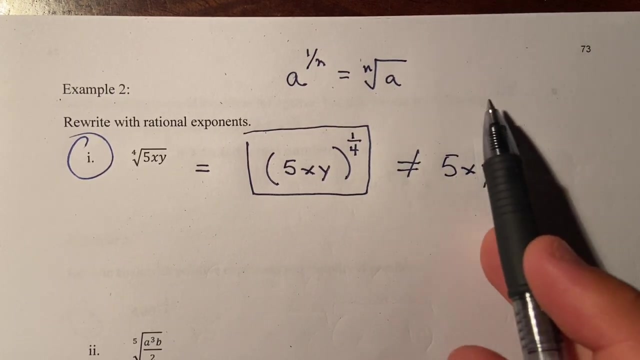 Since the entirety of 5xy is inside of the root, the entirety of 5xy needs to be under the power and in the parentheses. This is not equal to just 5xy to the 1-fourth in general. So this would be incorrect because it wasn't just the y that was under the fourth root. 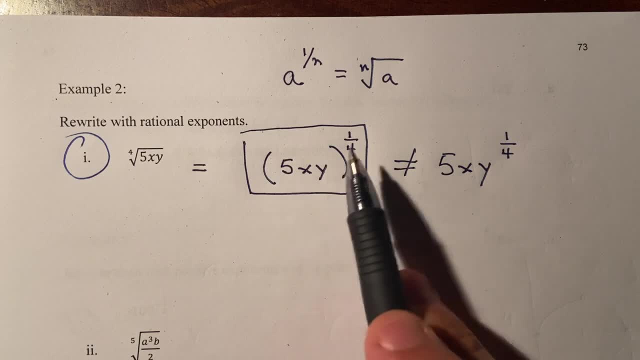 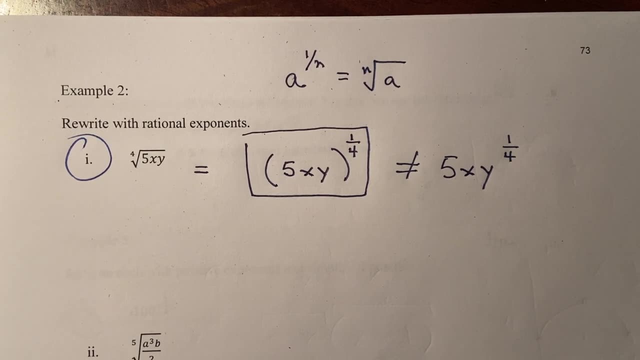 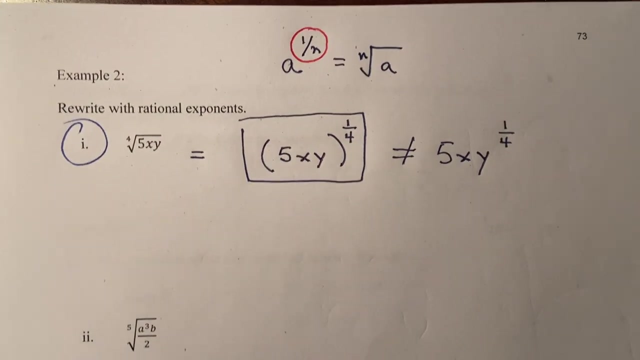 It's the entirety of 5xy, So these parentheses are necessary. Okay, so what we've seen so far is what we do with this type of power: Write a 1 over n At the bottom of page 73,. we're just kicking it up one slight notch. 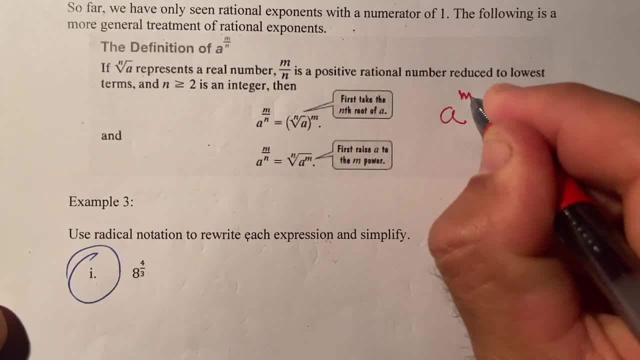 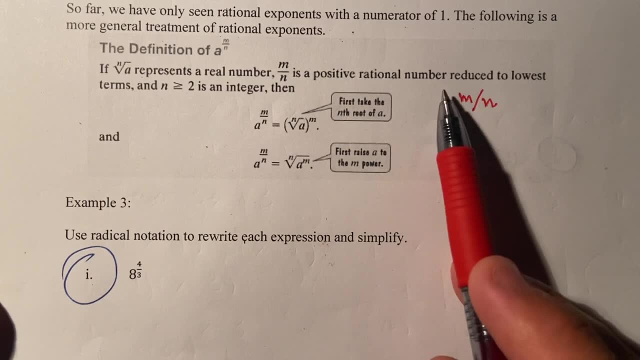 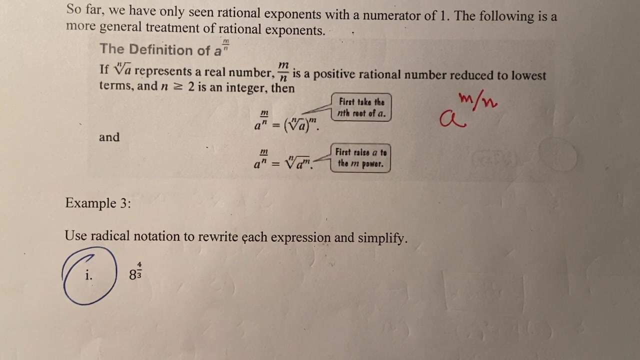 So just to zoom in on this thing, it says a to the m over n. So, rather than just working with a to the 1 over n, what if it was a more complex power like m over n? So this tells us what to do with that. 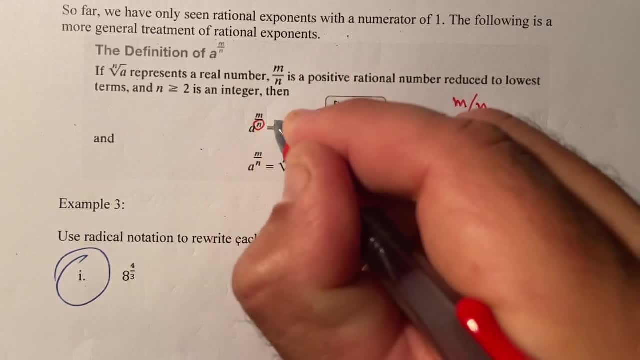 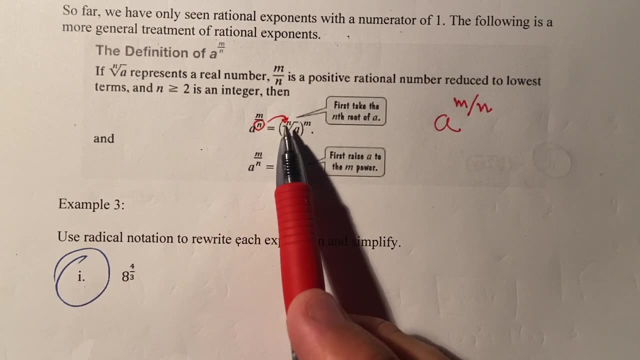 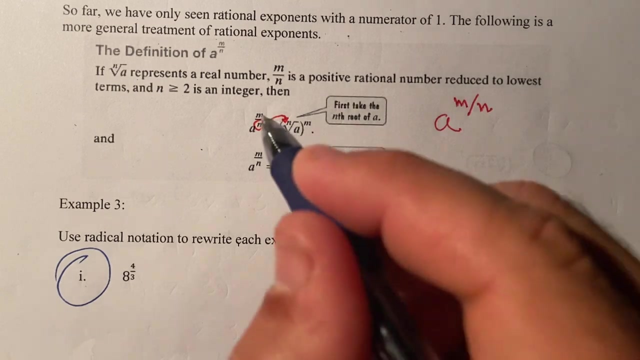 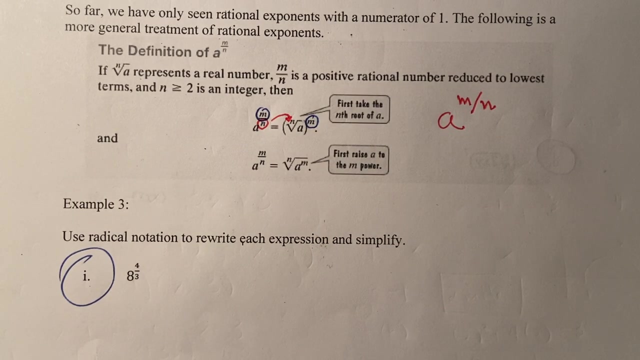 So still, The n is the type of root right. So the denominator of the power transfers and becomes the index of the root, the type of root. The numerator of the power becomes the power after the n-th root is applied. That's one option. 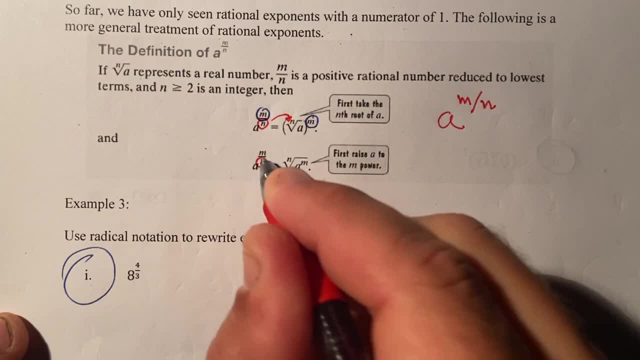 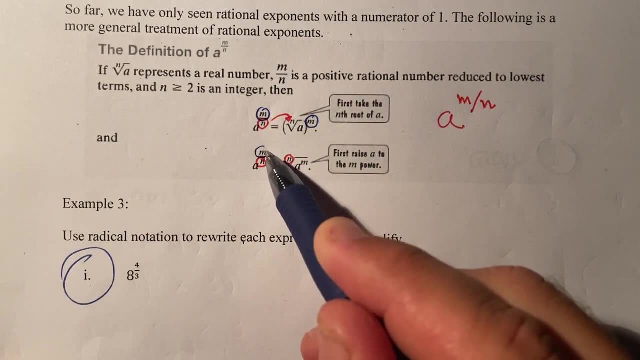 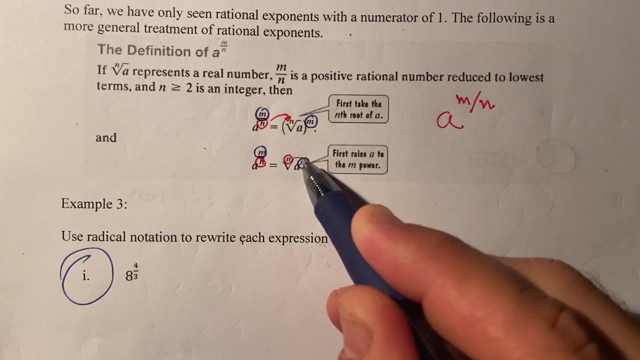 Another option, which is actually totally the same, Is you can have this n-th root still, And then you can actually, if you prefer, you can bring this m power- the one that's in the numerator of the fractional power- inside of the root. 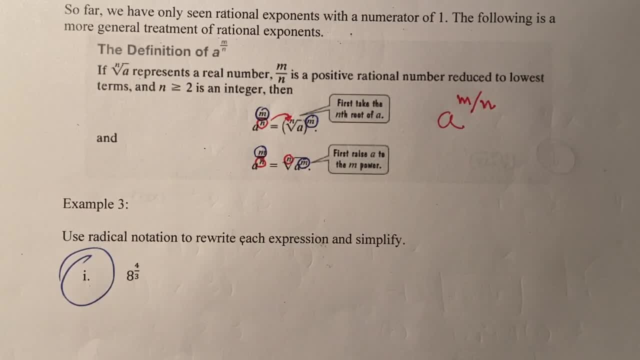 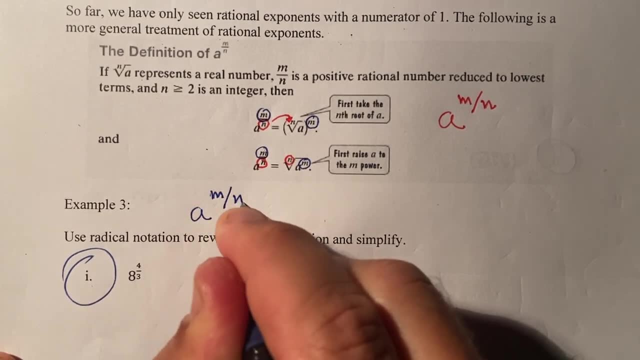 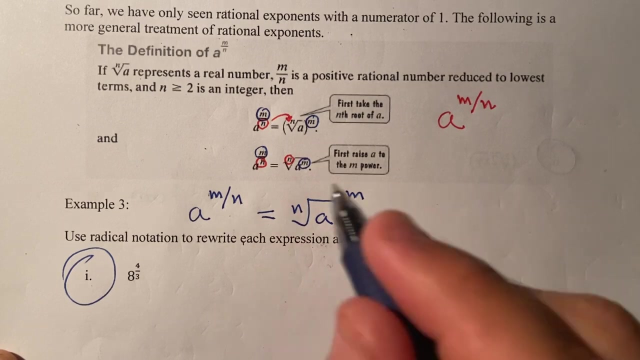 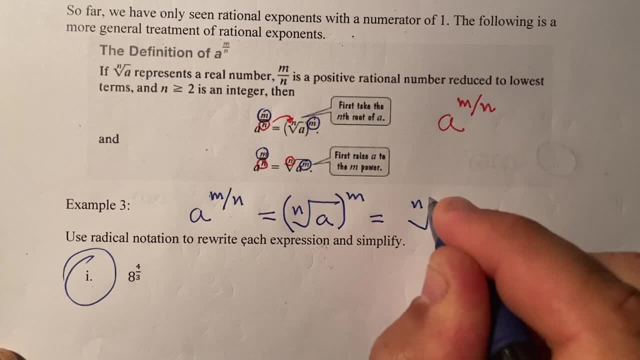 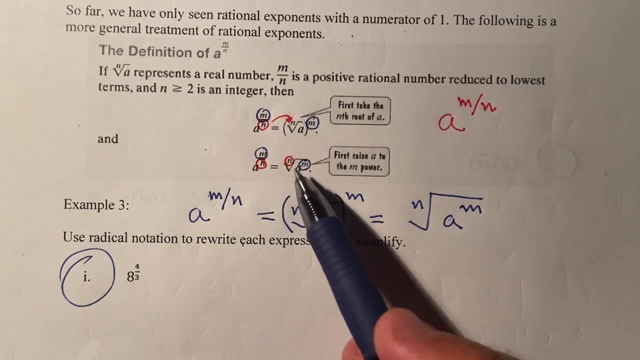 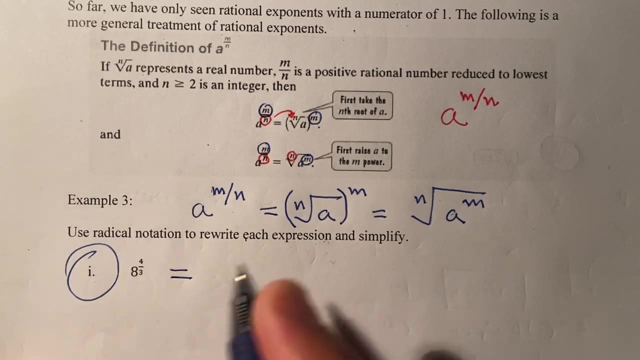 which is also equal to the n-th root of a to that power. So I'm just reiterating what's being said here. So you have options. So this thing would be equal to: Well, it'll be a cube, So this thing would be a cube root. 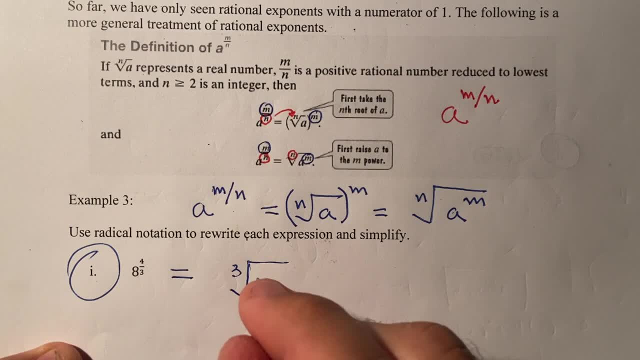 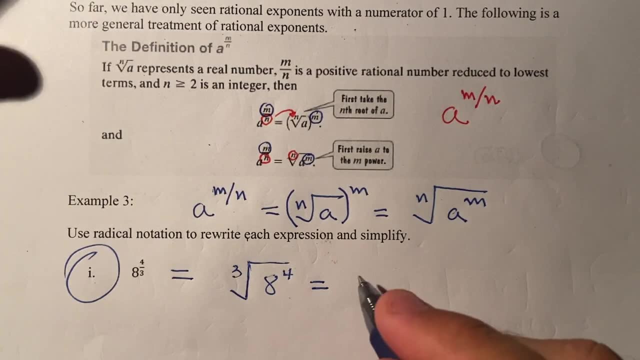 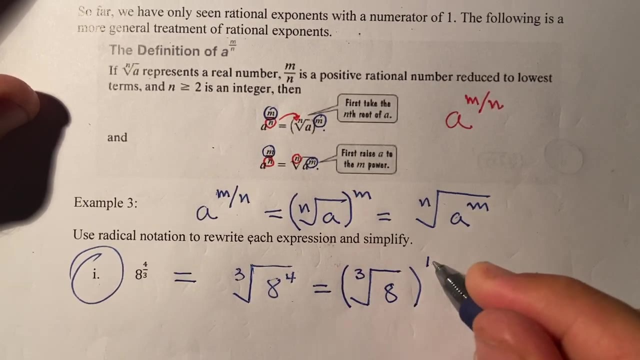 Right, That 3 becomes the type of root And then it'll be 8 to the 4th, Or I don't have to write both. I could think of this as the cube root of 8. And then, after I do that, I can raise to the 4th. 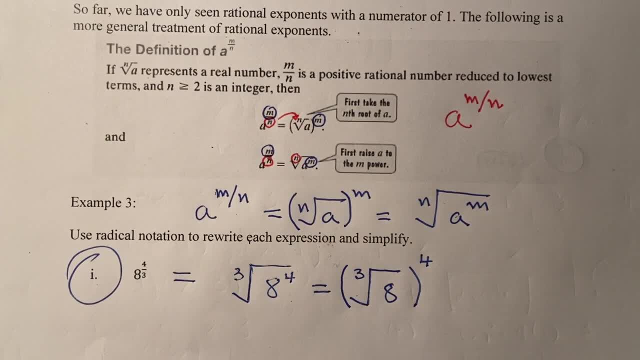 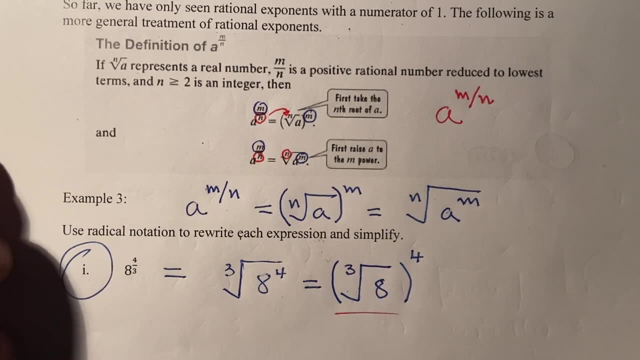 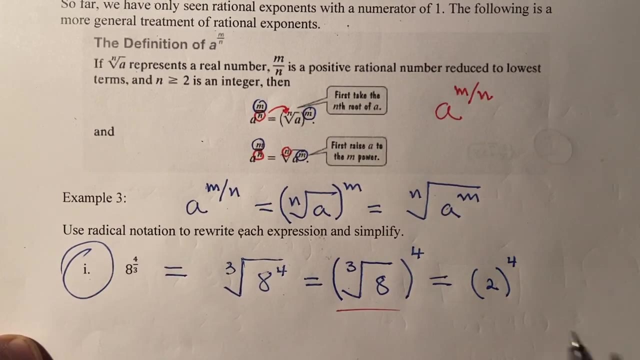 Both of these would be the same And that's what's written here. So for me at the moment I can do it easy this way, actually because I know the cube root of 8 is 2.. So I would just need to take 2 to the 4th. 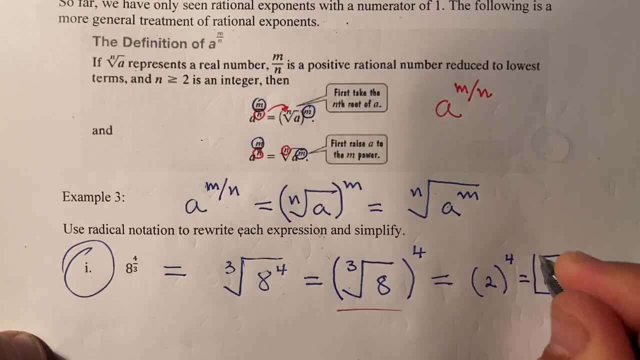 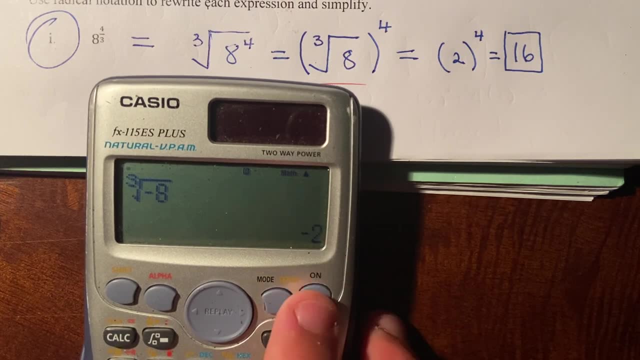 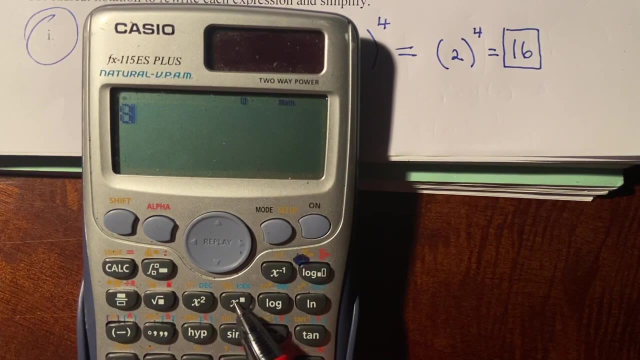 2 to the 4th is 16.. Right, If you want, though, don't hesitate to just use your calculator, So I could say 8 and then raised 2.. So this button, And I can just type it in as it was. 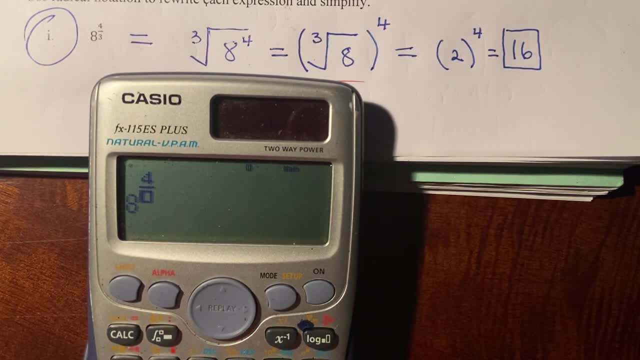 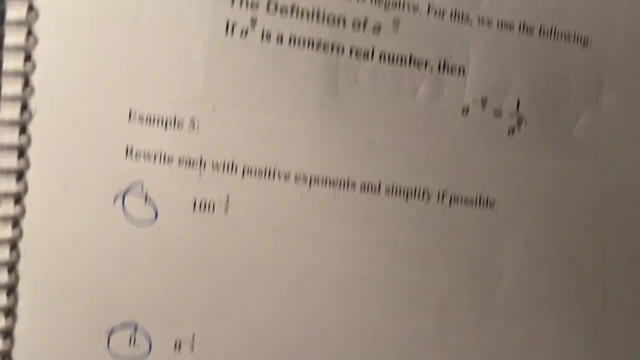 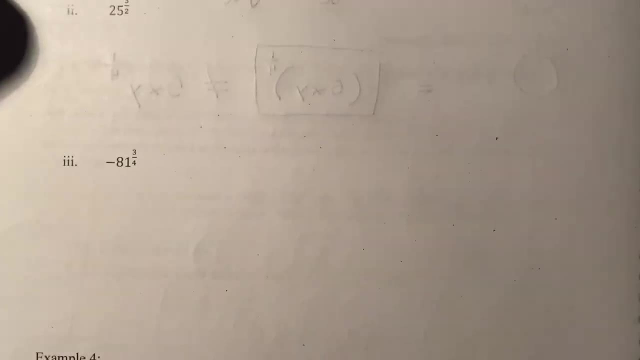 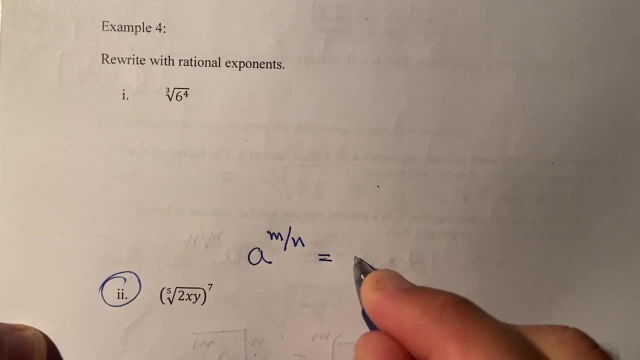 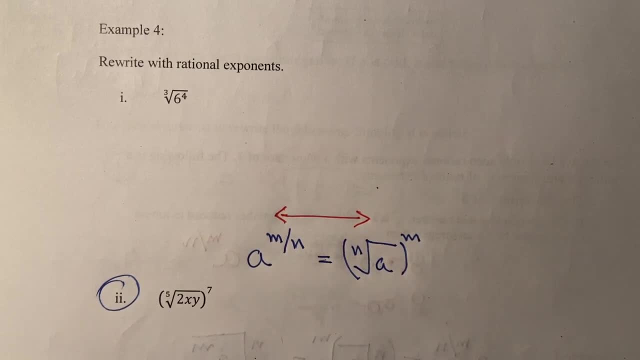 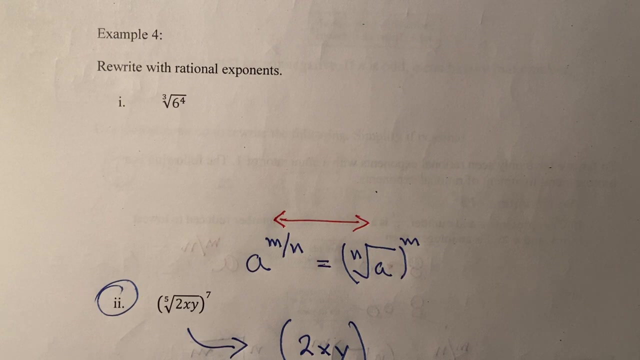 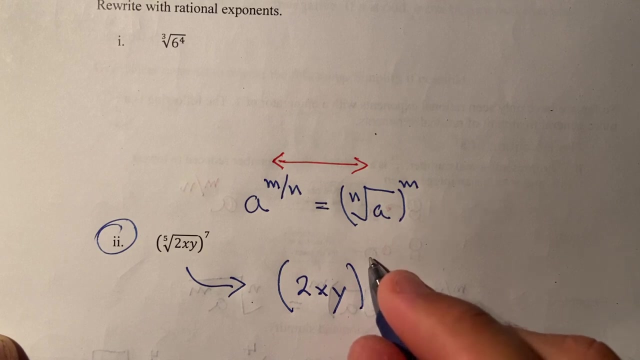 So we We're just going left to right, But it's also true to go right to left. So this one, we would have 2xy inside of parentheses and it was a fifth root. so that's the type of power as far as the 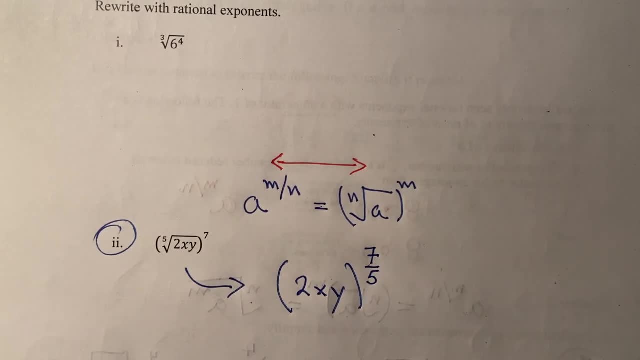 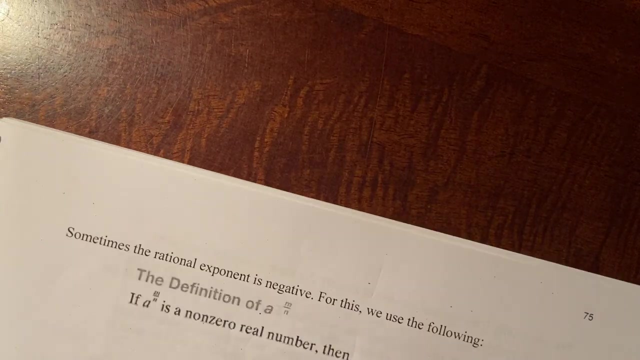 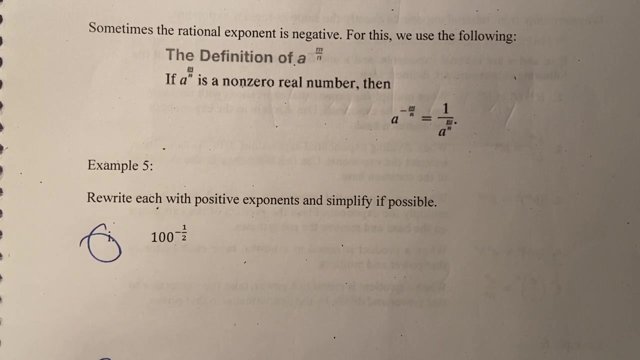 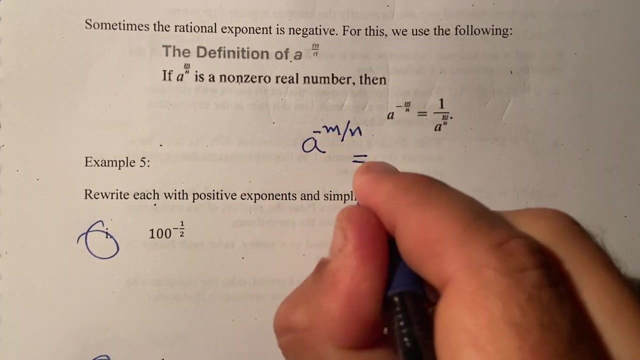 denominator goes, and then the seven goes up top right, so that five is the denominator, that seven is the numerator. so what about negatives? so that's one type that we haven't talked about yet. so what this is saying is, if you have a to the negative, n over n, then that's. 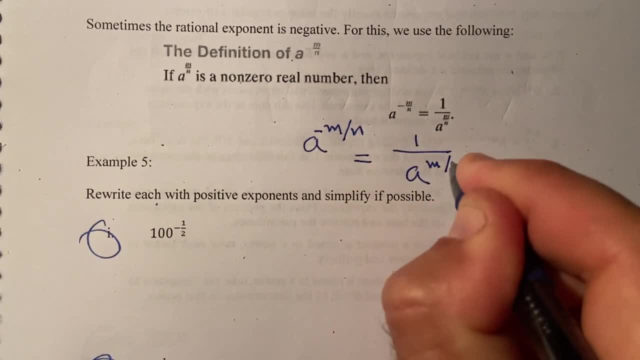 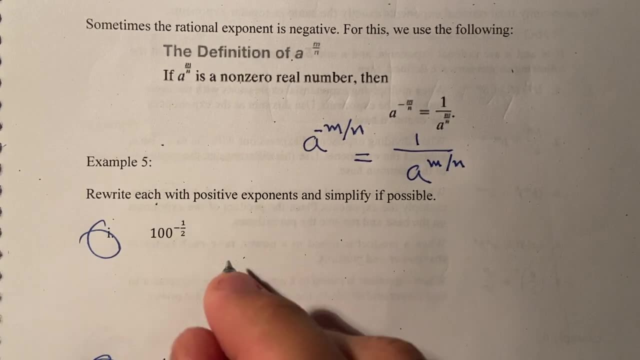 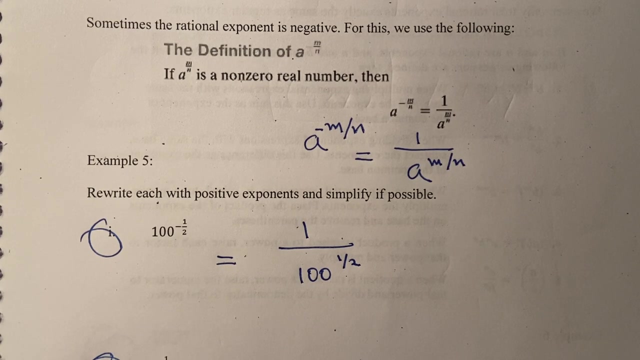 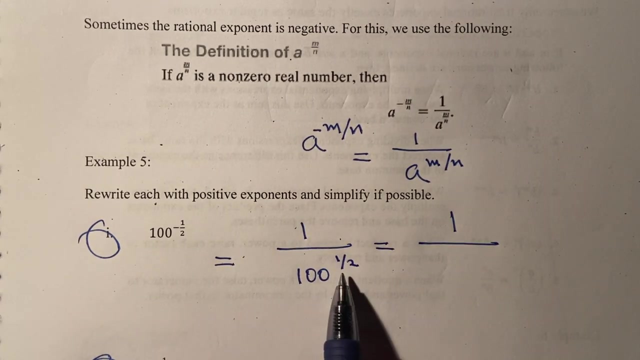 actually the same as 1 over a to the positive, n over n. so if I have a hundred to the negative one half, this would be the same as one over a hundred to the positive one half. the square root can be written. we have a one-half power so I can write that as a. 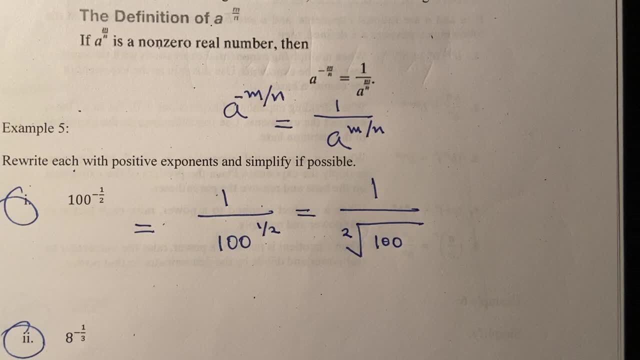 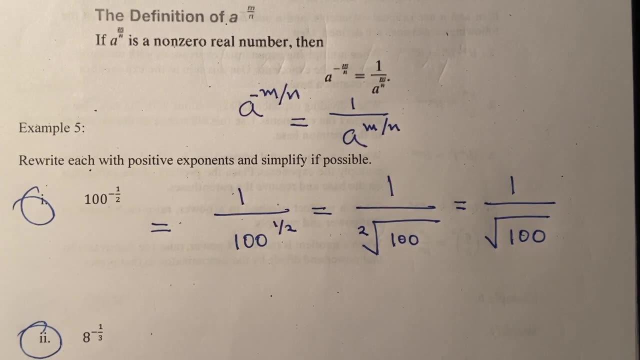 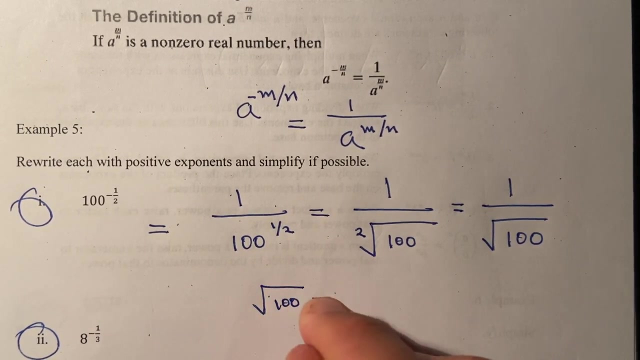 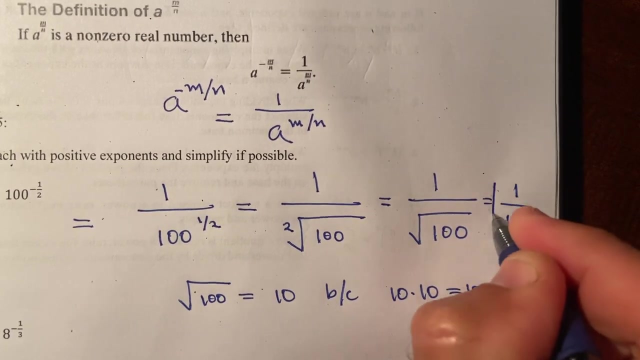 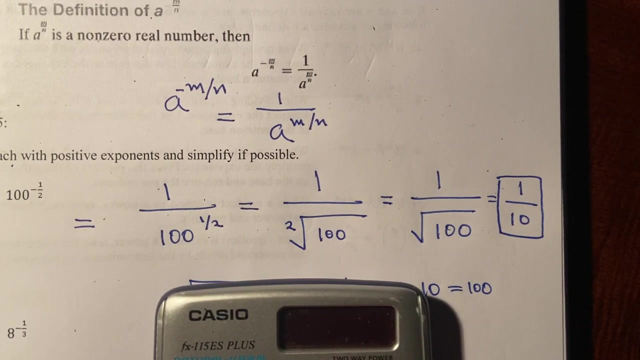 square root of 100. for square roots, we typically don't write that too, so this would be the same. and I know the square root of 100 is 10, because 10 times 10 is a hundred, so I can write one. don't let me stop you from using your calculator as usual. so 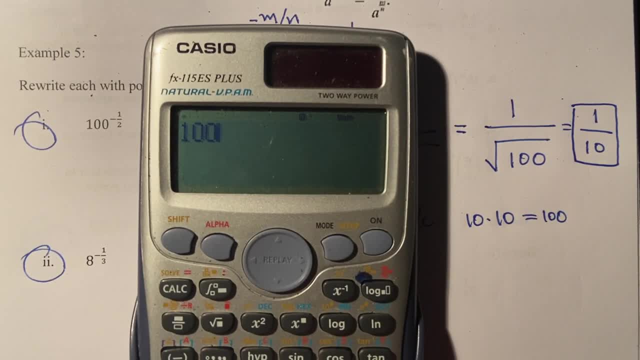 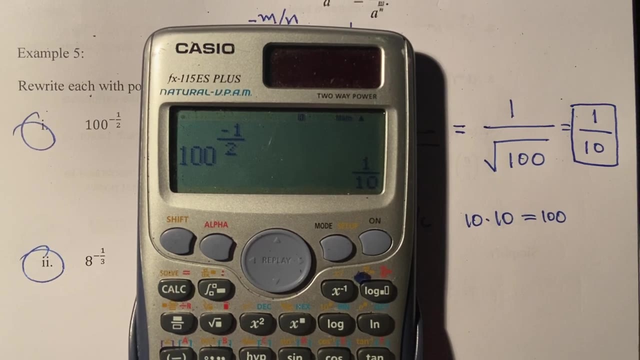 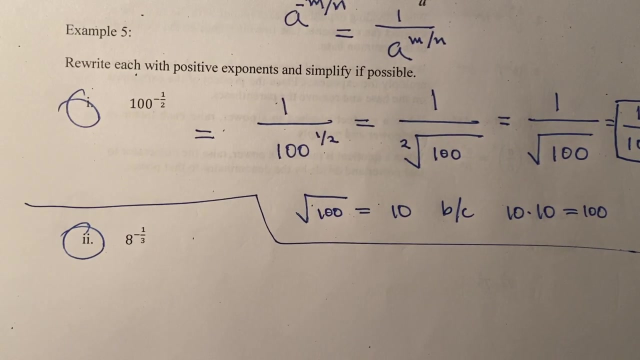 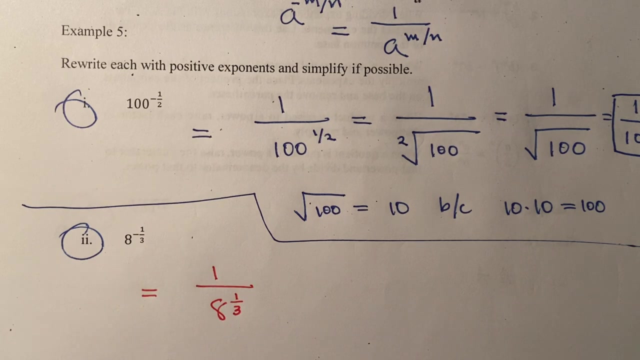 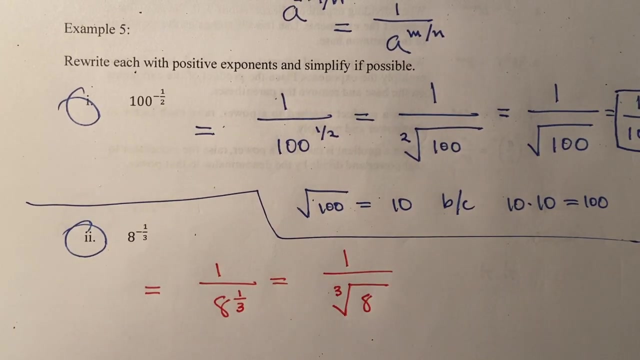 hundred- the power was right here- and then the fraction. so negative one half equals 10: 8 to the negative 1: 3rd. we have 1 over 8 to the positive 1: 3rd. that would be the same as 1 over the cube root of 8. 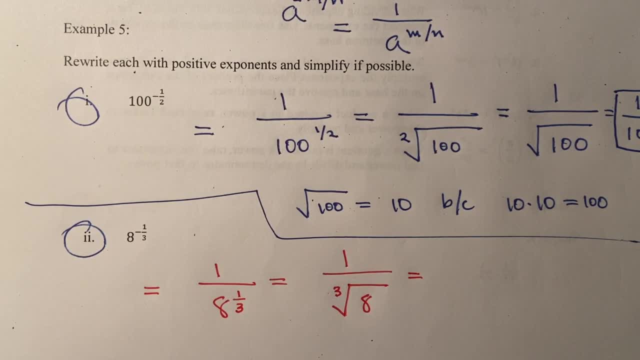 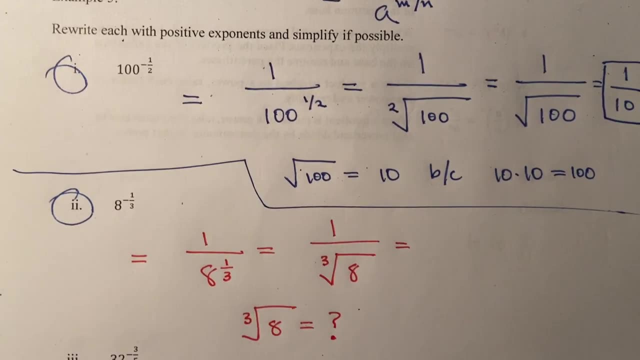 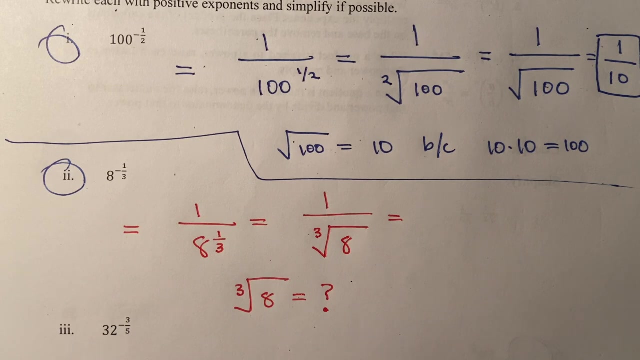 the cube root of 8 means we're looking for a number, So let me write this down if you're having trouble with that. So just imagine we're unsure of what. this is The definition of any root. in this case, we have a cube root of 8.. 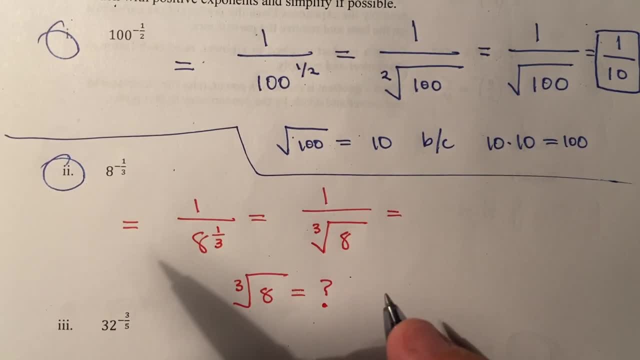 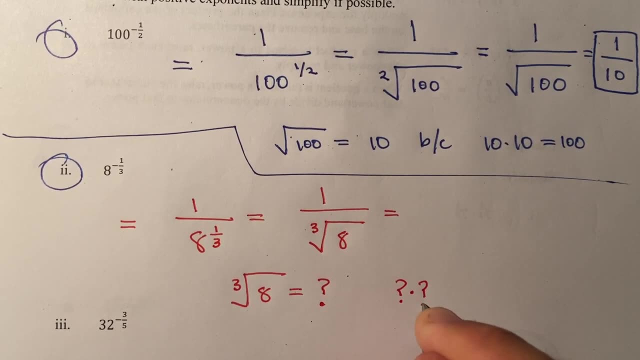 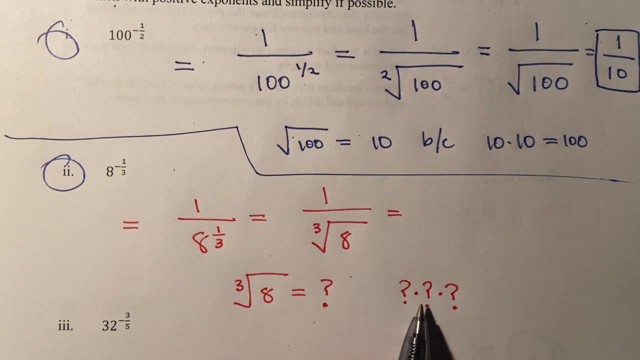 So what we're trying to do for that is, we're looking for a number times itself, 3 times, right? so whatever number this is equivalent to will be the number, such that multiplied by itself 3 times. based on that, 3, equals 8.. 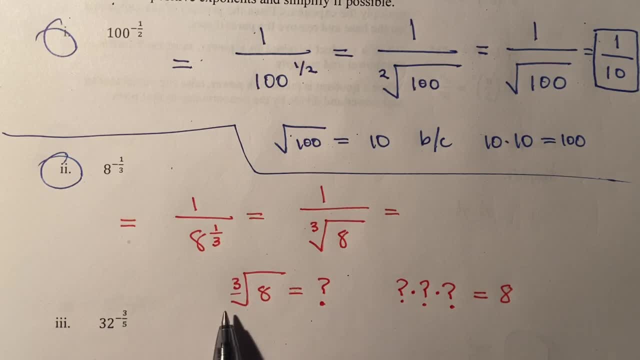 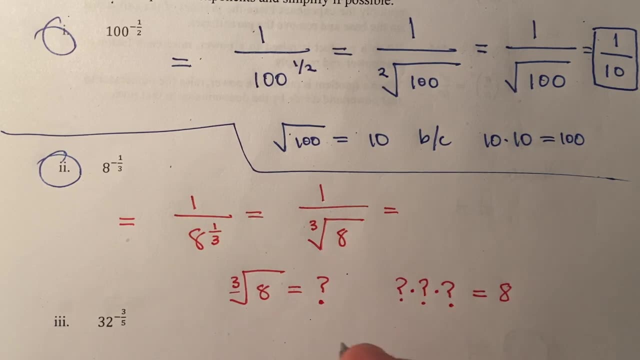 This is the kind of puzzle we're looking for when we're presented with something like this. So for that reason, question mark equals 2, right. 2 times 2 is 4.. 4 times another 2 gives us 8.. 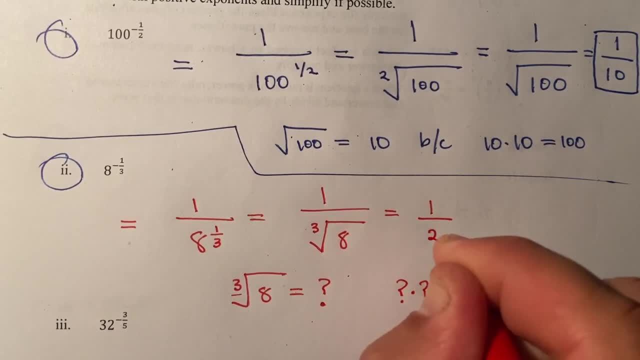 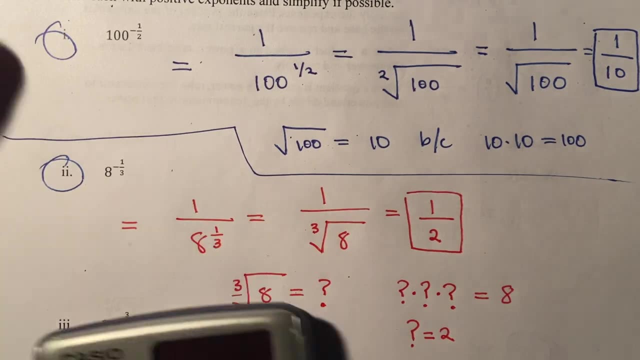 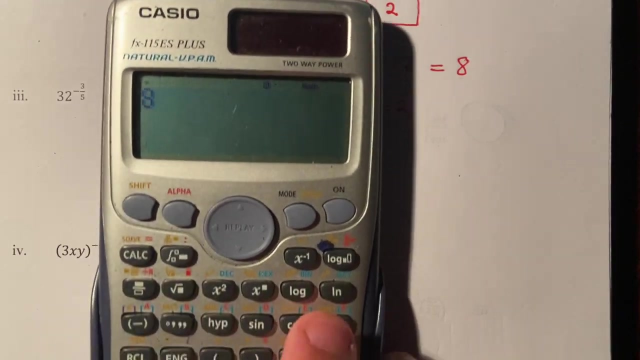 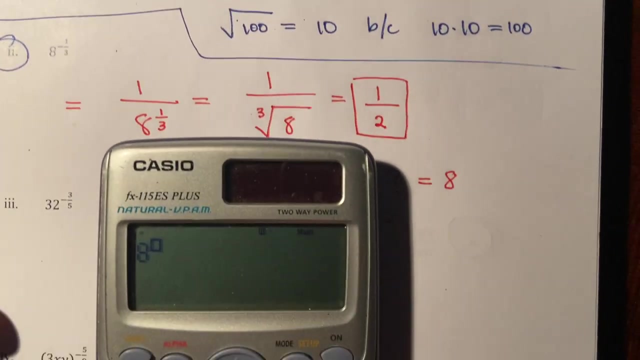 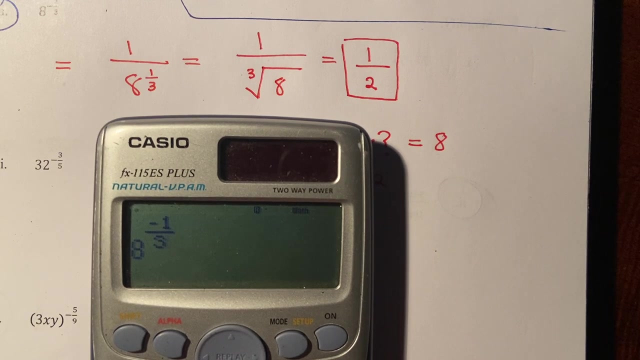 So I know the cube root of 8 is 2.. In other words this is 1 half. So 8 raised again is this button Fraction, And then negative Negative 1 third. There's that 1 half. 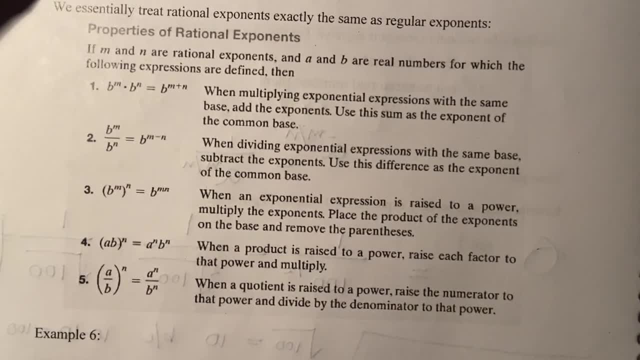 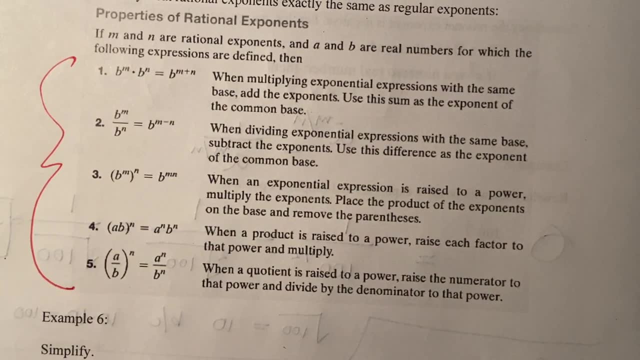 So yeah, on page 76, there's a bunch of these power properties. You're going to want to get to know these All five of them. Okay, so this first one says: if you have the same base and those are raised to powers. 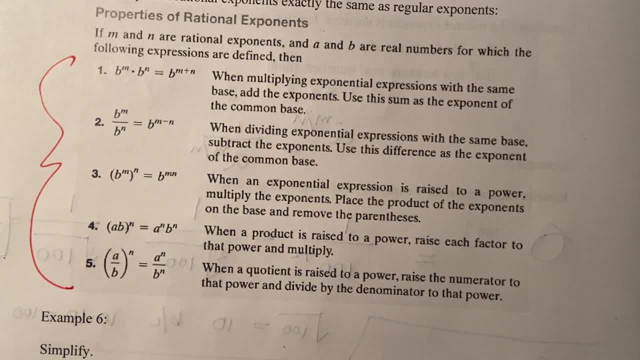 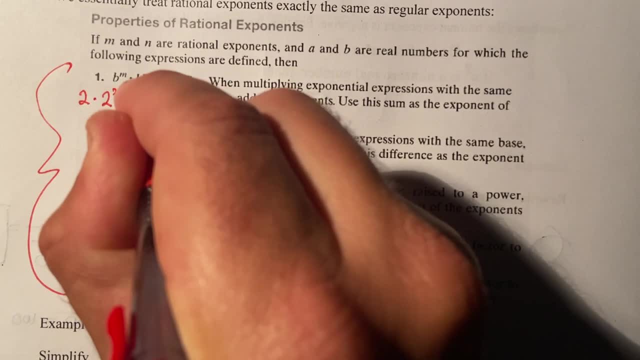 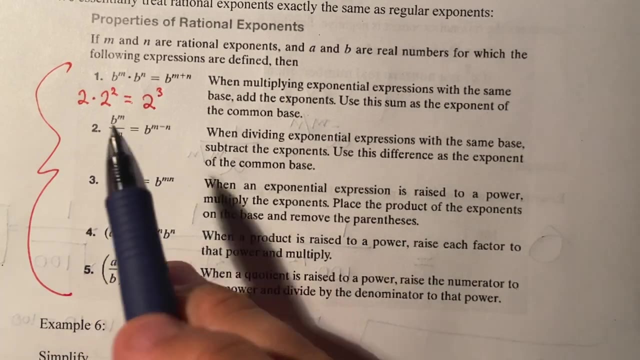 that you actually add the powers. So, for example, if you have 2 times 2 squared, that would be the same as 2 cubed. Number 2 is similar If you have b to the m divided by b to the n. 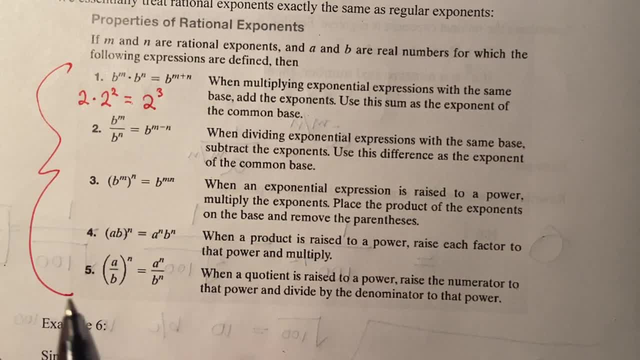 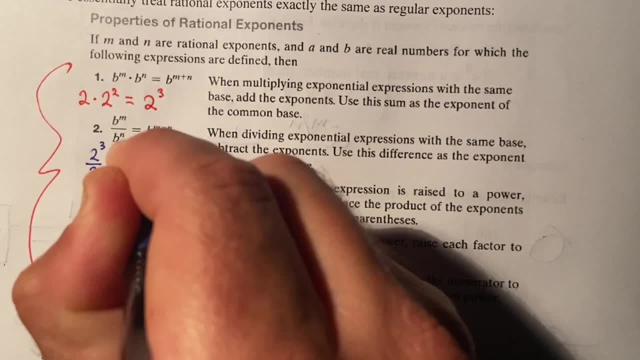 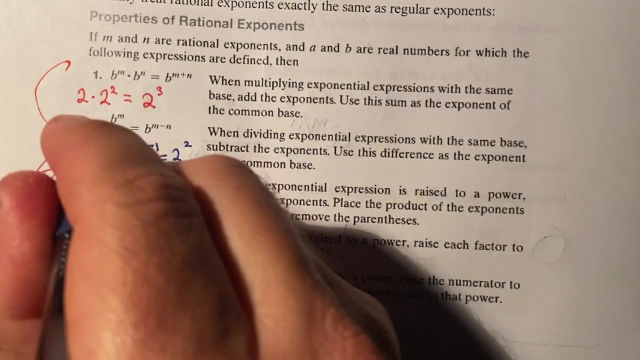 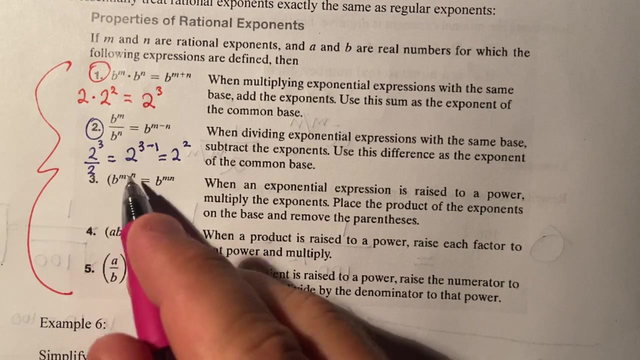 then you're actually subtracting. So if we had 2 cubed over 2, then that would be the same as 2 to the 3 minus 1, or 2 squared b to the m to the n, If you have 2 cubed to the 4th. 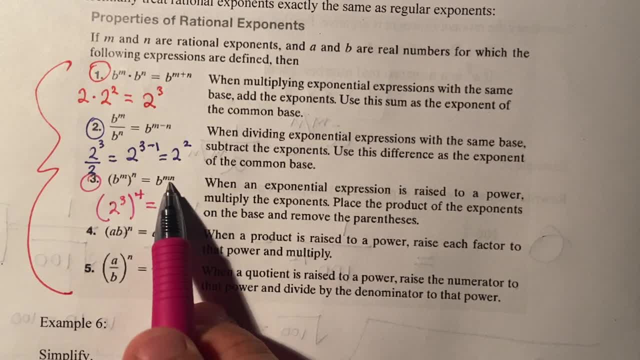 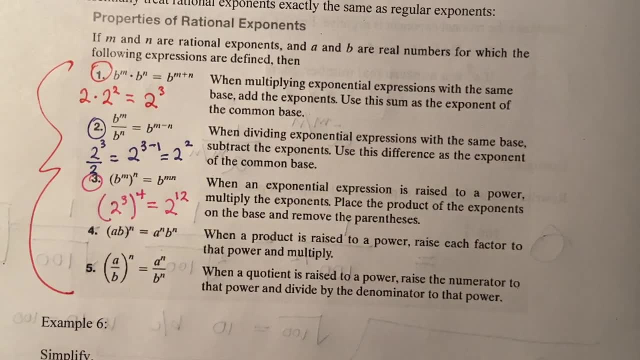 then if you have powers to powers, what this is saying is you actually multiply those powers. So this would be 2 to the 3 times 4, in other words, 2 to the 12, and so on. So we're going to get practice working with these. 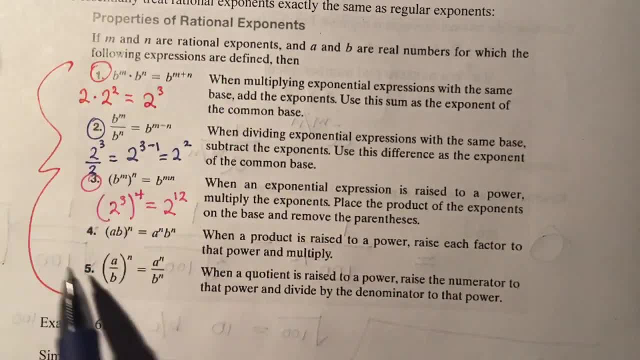 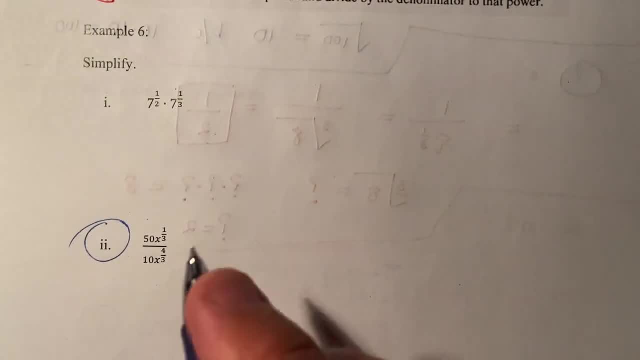 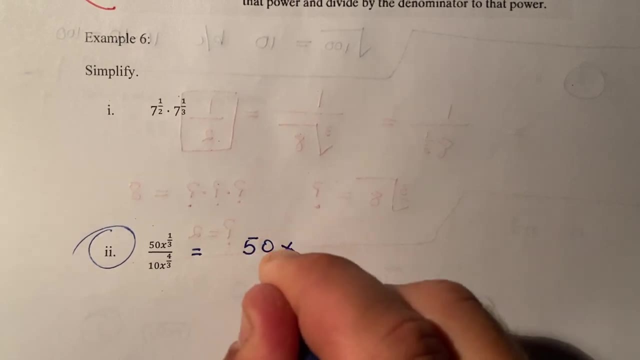 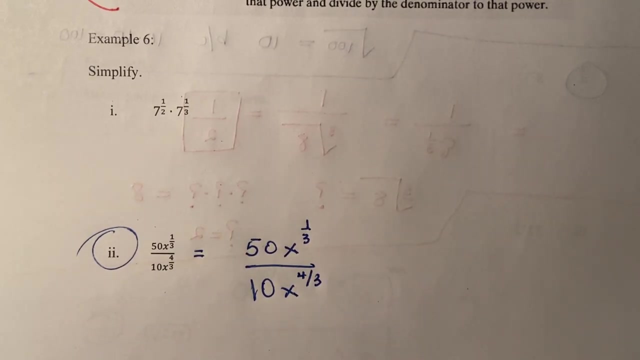 And you do want to just get enough practice to where you just ultimately know these. So example 6, we have 50x to the 1 third Over 10x to the 4 thirds. So it says: simplify, So 10 goes into 50 five times. 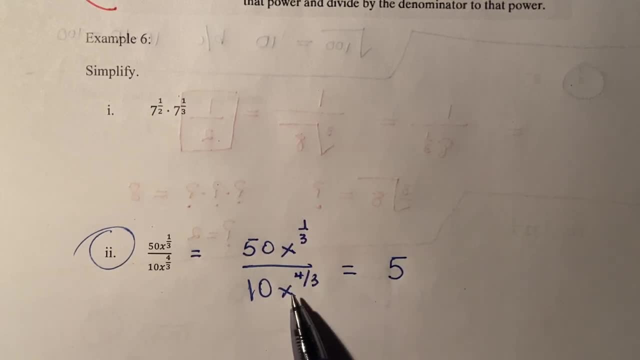 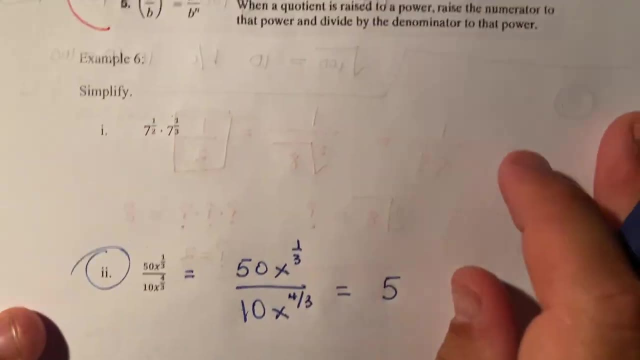 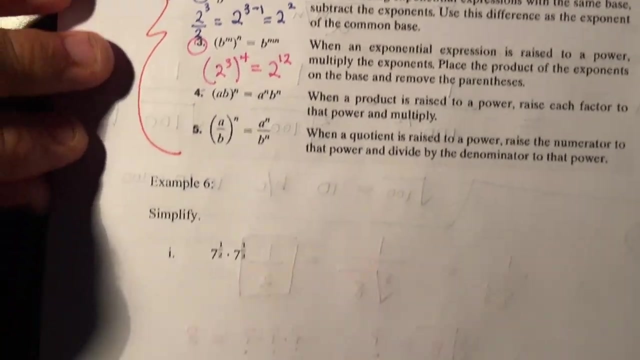 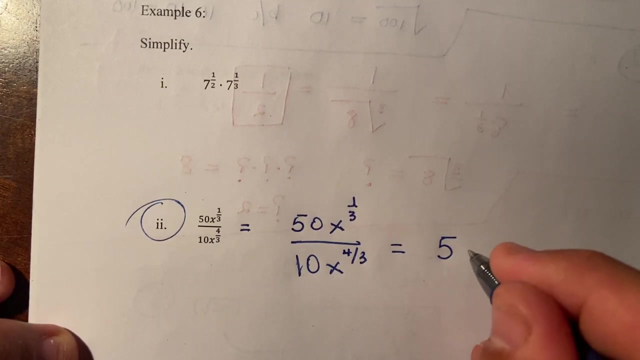 So I can simplify that. And then I have x to the 1 third over x to the 4 thirds. That's reminding me of number 2 up here. In this case we have x instead of b, So what this is suggesting is I can just take 1x. 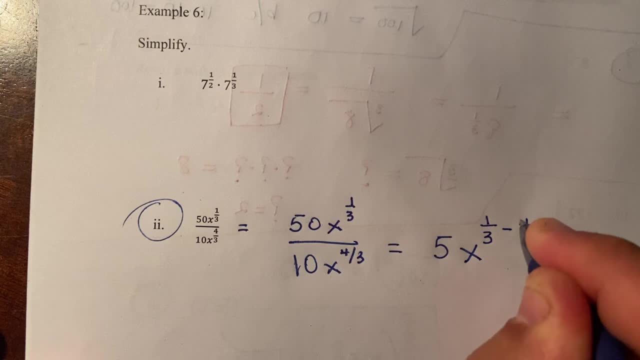 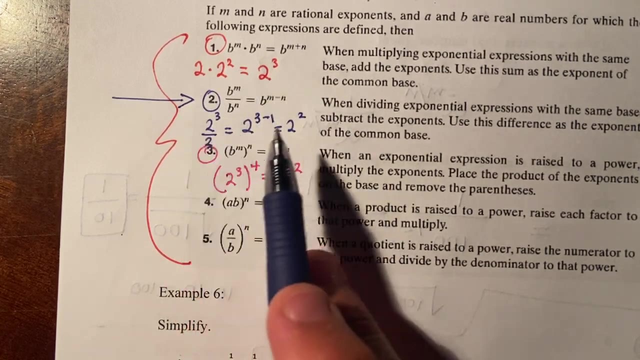 and go to the 1 third minus 4 thirds, And so I'm applying the second property right, The upper power minus the lower. So here's the power. I'm going to do that, I'm going to do that. I'm going to do that. 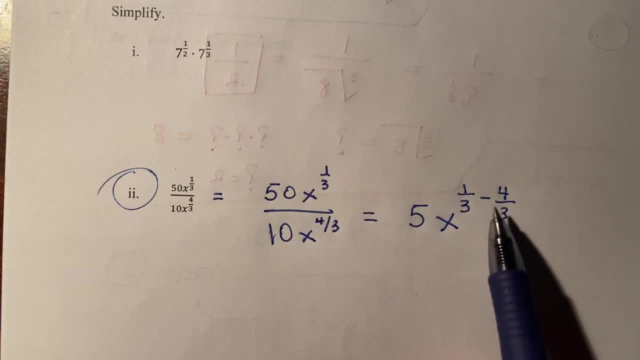 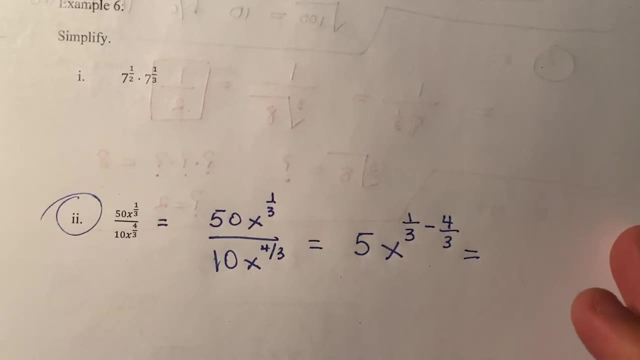 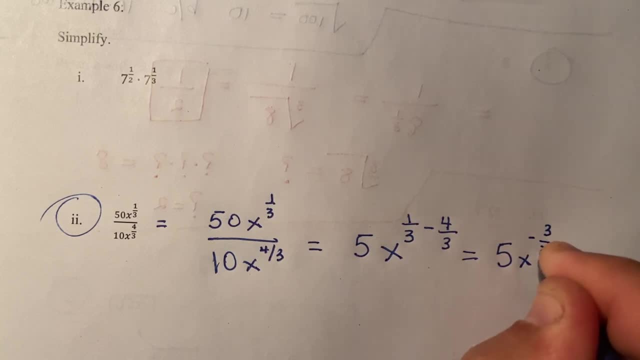 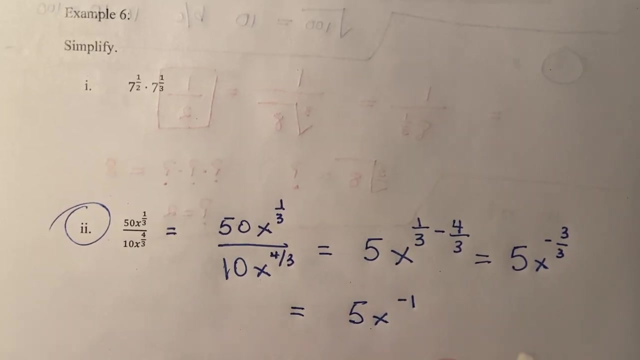 We'd have 5x to the negative 3 thirds. right, 1 third minus 4 thirds gives us negative 3 thirds And that would be equal to 5x to the negative 1.. and from the property on the previous: 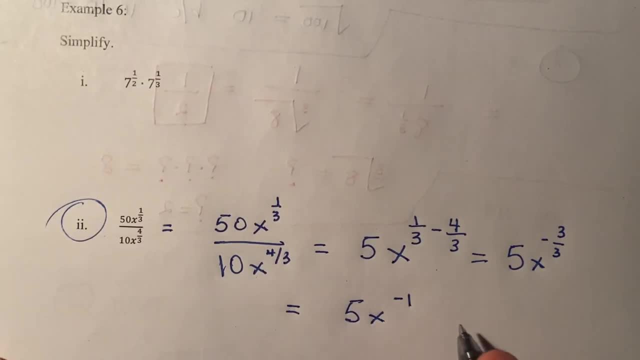 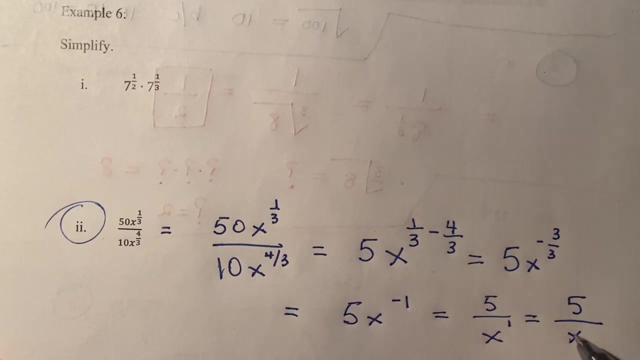 page yep, on page 75, the negative power can be rewritten in the denominator as a positive power, And with a power of positive 1, we usually don't write that 1. So I'll just leave this as 5 over x. 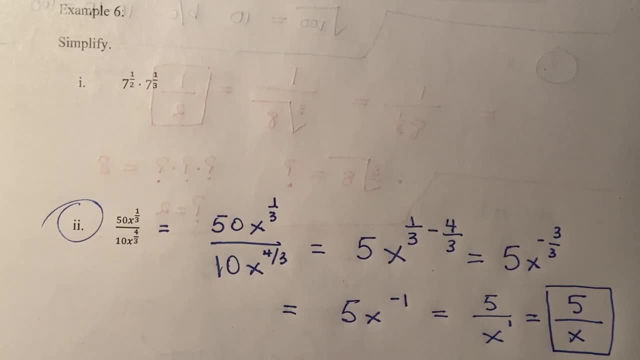 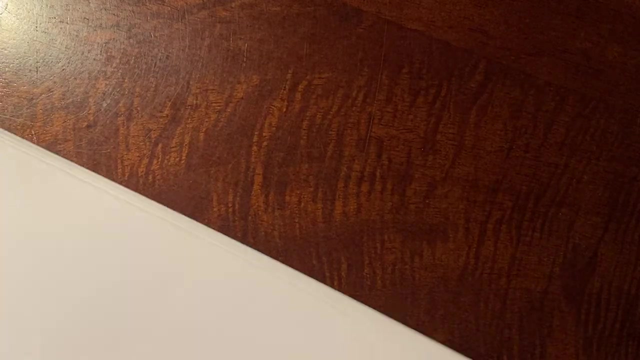 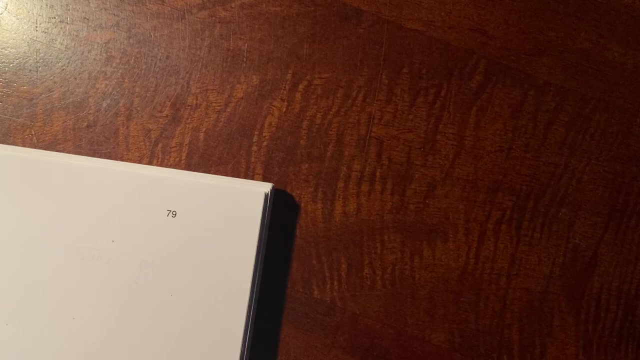 The calculator can't do this one, by the way, because it's algebraic, right? This calculator is great at arithmetic, but it's not going to be able to help us simplify this. Alright, 77.. You'll see that I pick it up on page 78 in a 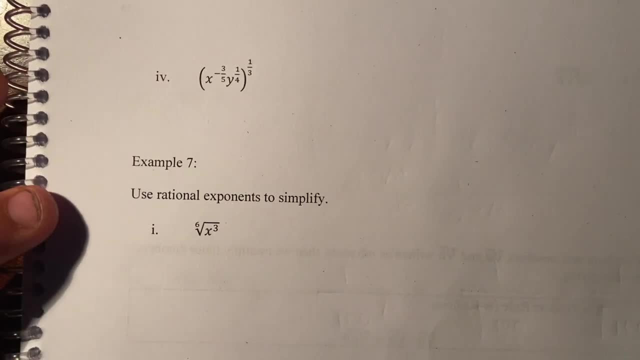 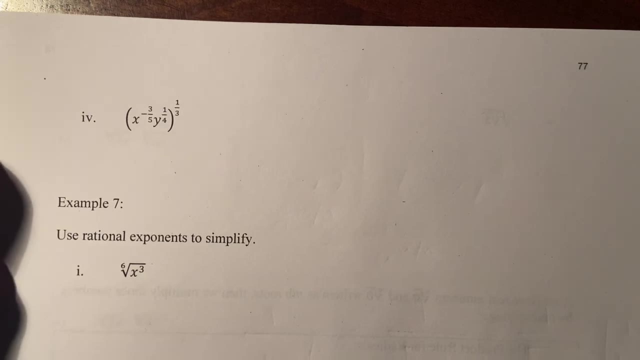 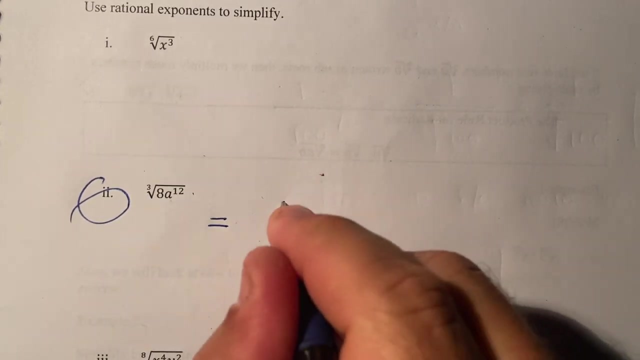 separate video. Okay, so I'll just do a couple more. This is page 77.. And just a couple more simplify cases. So I'll go to part 2, actually. So we have a cube root. That means this entire thing. 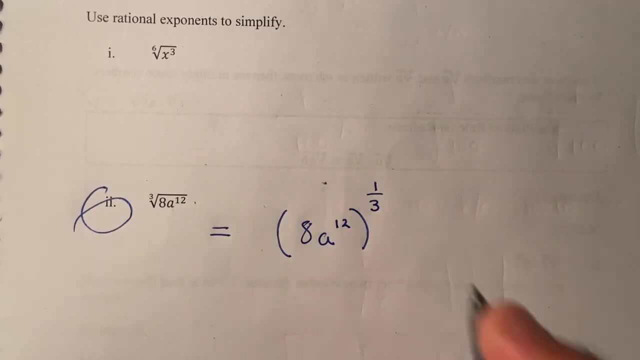 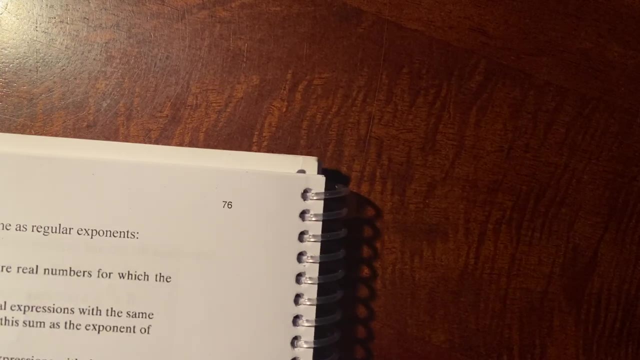 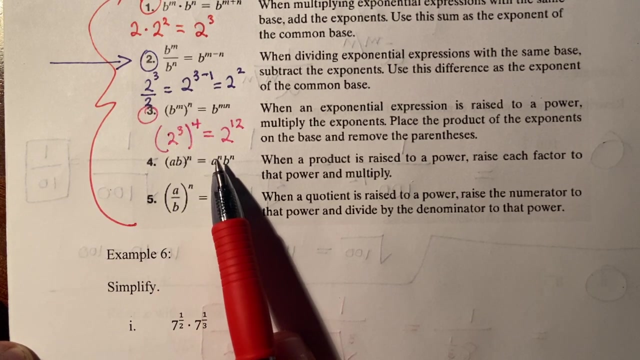 8a to the 12th needs to be raised to the 1 third power. One of our properties on the other page said if you have a product raised to the nth power, that every member of that product takes on that power. 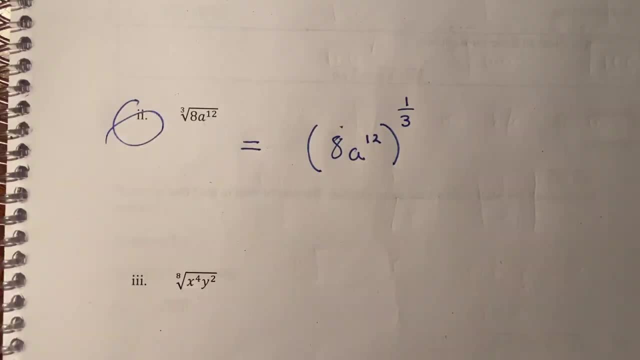 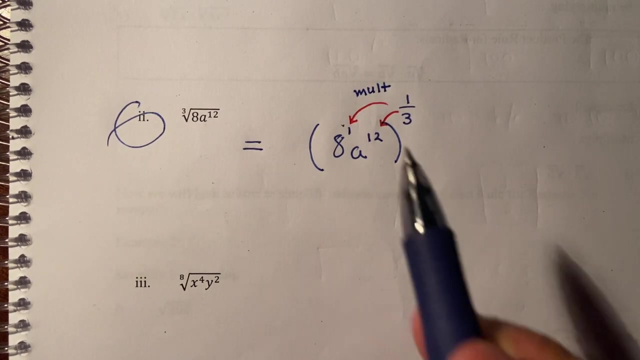 Okay, so for number 4. there, I see that everybody in here needs to take on this power, And not only that, when they take the power on, it comes in through multiply. So what I'm going to do is I'm going to take a to the 1th. 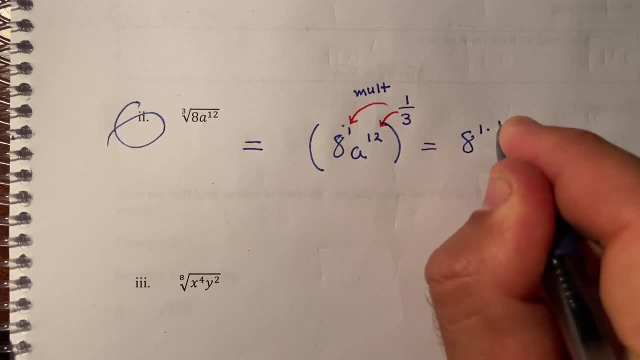 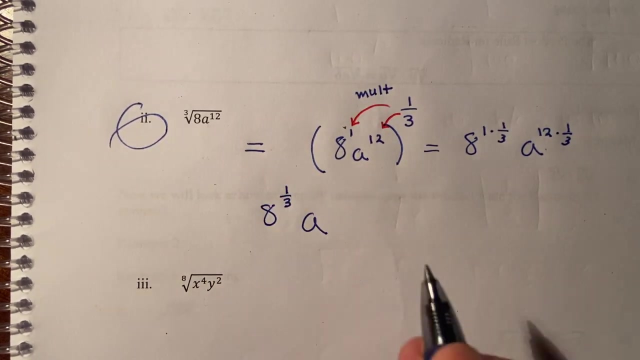 times 1 third, and then a to the 12th times 1 third. So I get. well, let me write 8 first, so I just get 8 to the 1 third times 12, times 1 third is 4.. So I'd have a to the 4th. 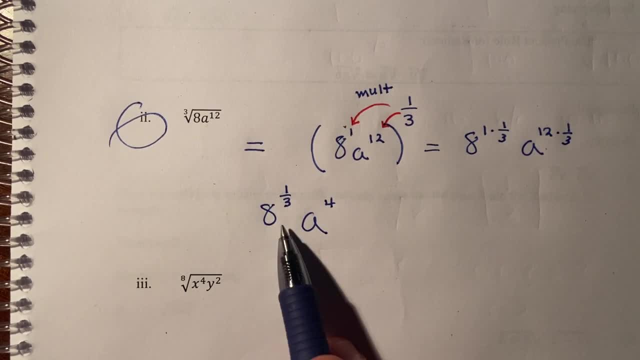 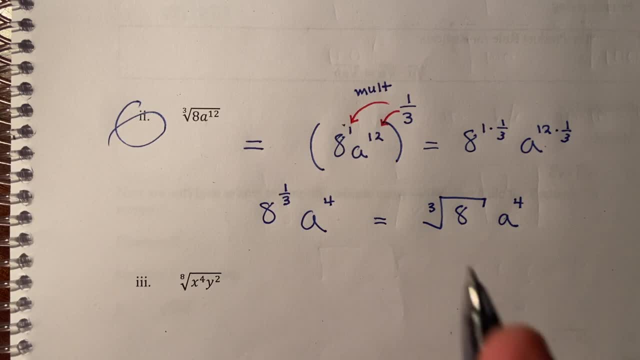 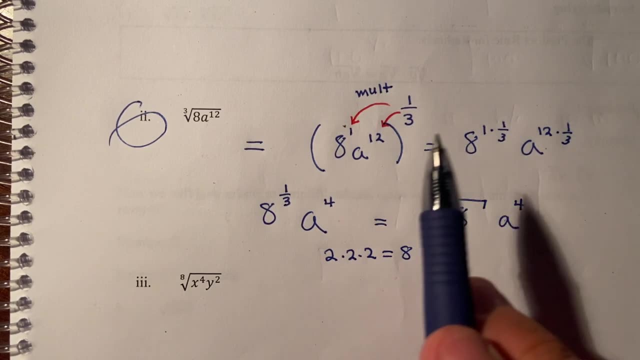 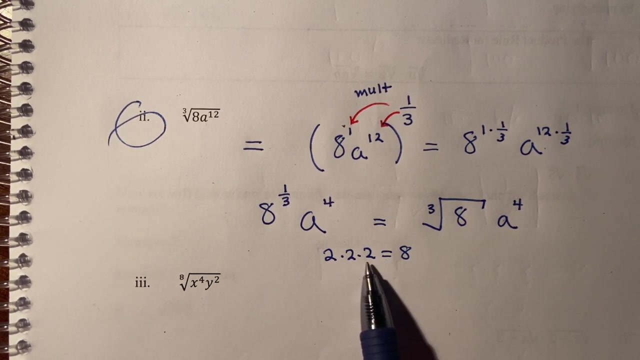 And I know that the cube root of 8 is 2, because 2 times 2 times 2 is 8.. So that's basically what a root means is: if you have some nth root of a number, you're looking for a number that multiplies that n times to produce this number here. 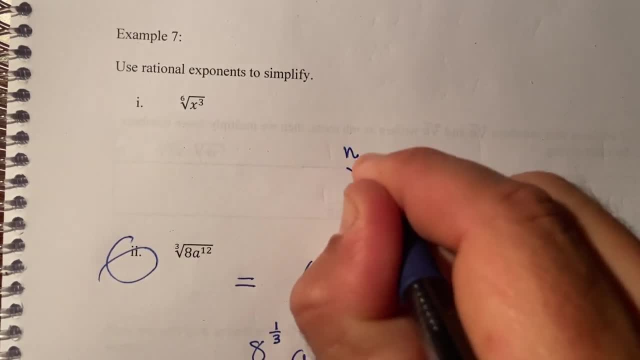 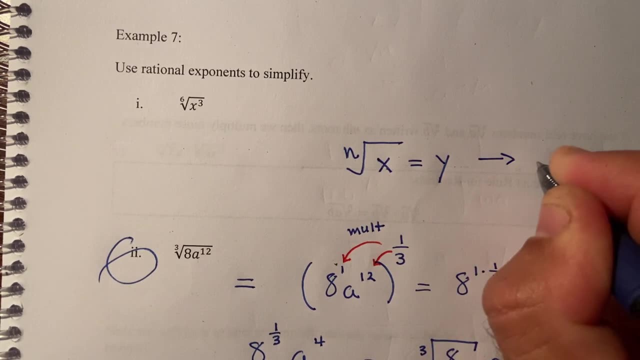 Okay. so just to summarize, if you have the nth root of x equals some number, y, and that means y times, y times, dot, dot, dot y n times. and then you have the nth root of x equals some number, y times y times, dot, dot, dot y n times. 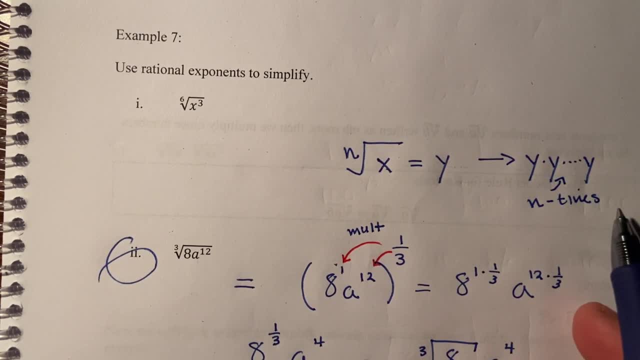 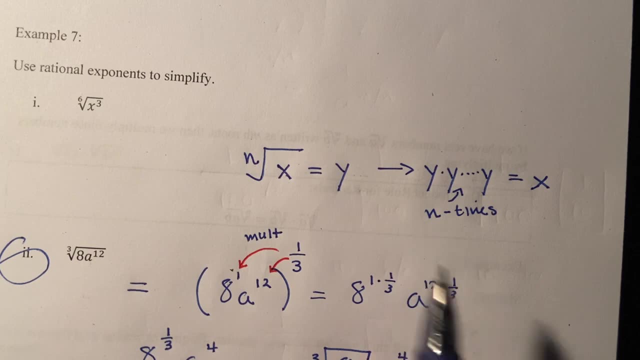 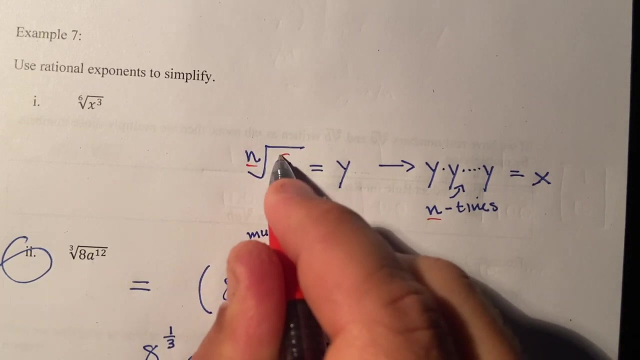 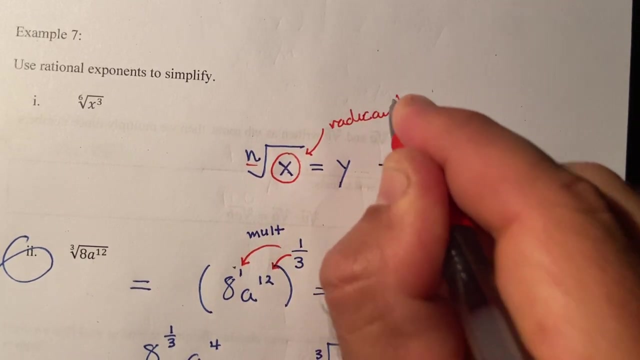 so n multiplications. this would mean you multiply up to x, So this n tells us how many times to multiply. This x is actually called the radicand, And that's what we're trying to multiply to, And this n is called the integral. 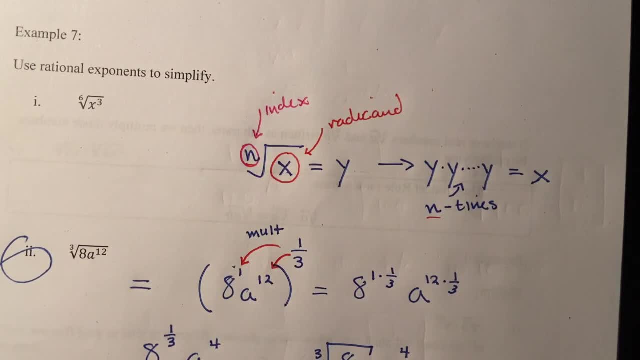 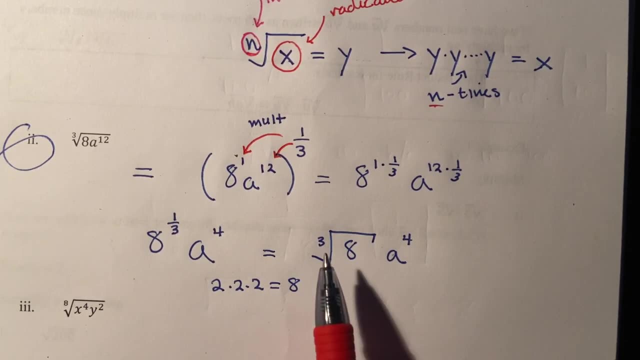 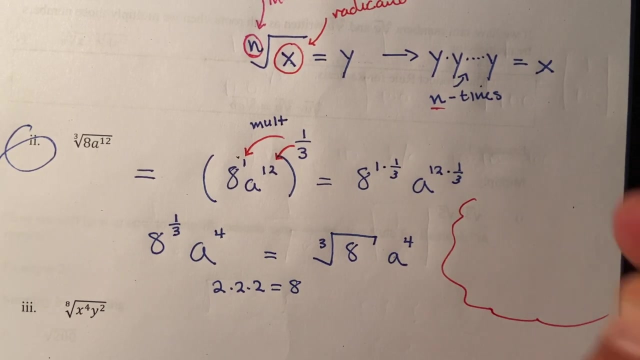 And that's how many times we multiply. So in particular, here I have the cube root of 8.. If that's some number, maybe you're thinking about it. Let's just say it equals y, Like you don't know what it is yet. 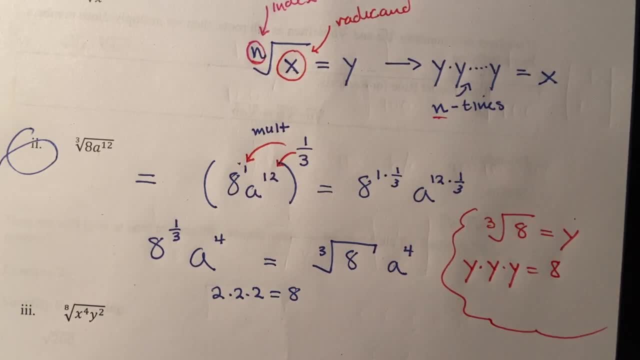 y times y times y would need to equal 8.. So that 3. It means we're multiplying 3 times and we're multiplying to try to get 8. So this implies that this should be a 2. So I can simplify this piece. 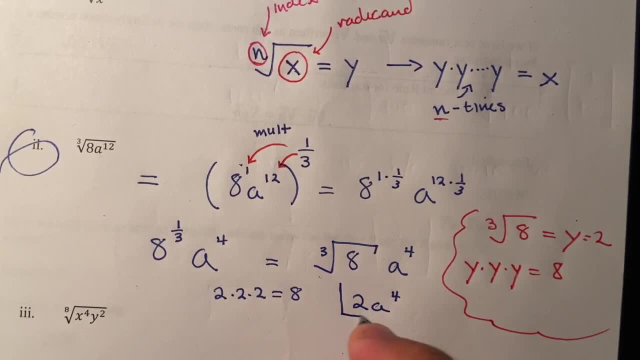 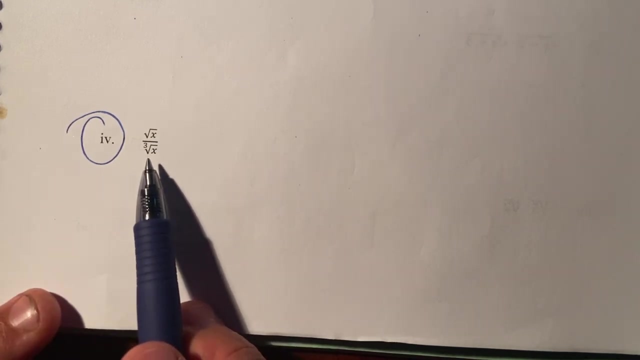 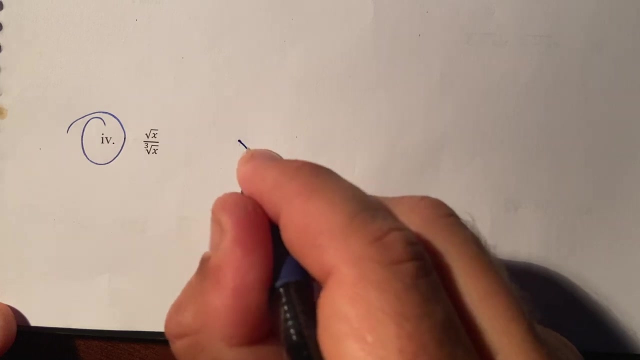 We should just have 2a to the 4th. That's the exact same as this thing. Okay, Maybe one more. Part 4, we have the square root divided by the cube root of x. Okay, So the square root of x can be thought of x to the 1 half power, right? 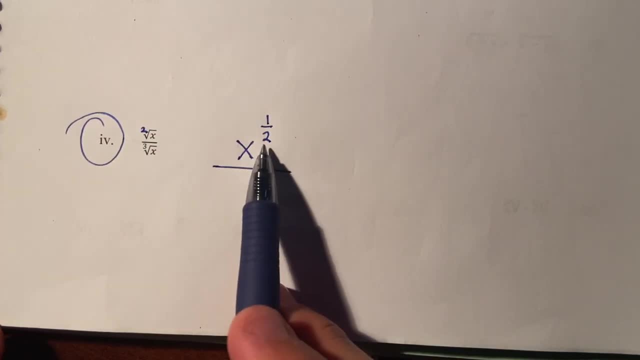 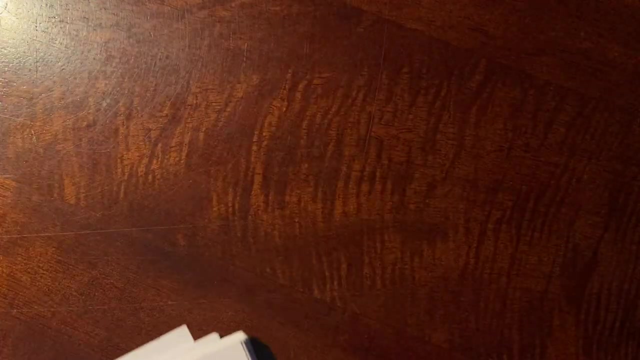 This index gets transferred over here as the denominator of the power And then this cube root of x can be thought of as x to the 1 third. So this is one of your power rules. I'm calling them. They're really exponent rules here on page 76.. 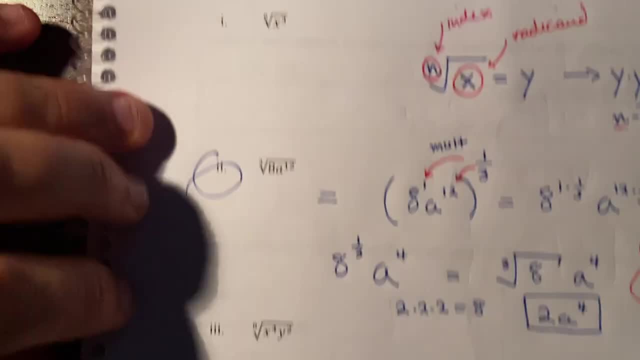 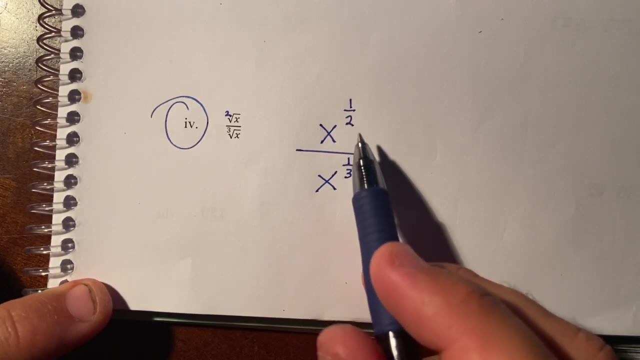 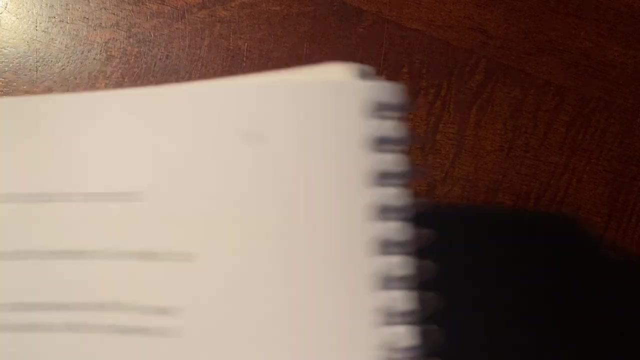 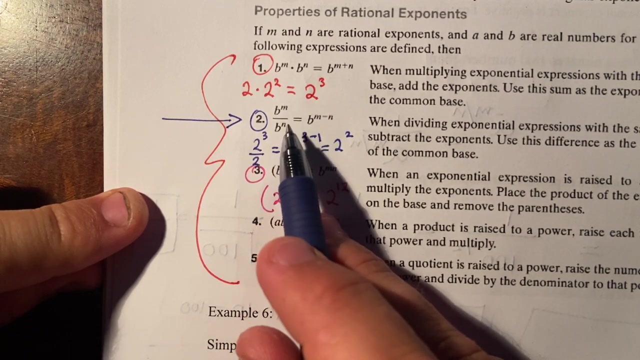 So one of these is helpful at this point: When you have the same base, two powers, we can subtract the upper minus the lower. So based on, I think, it's number, let's see number 2.. It's this one again, same base power, power. 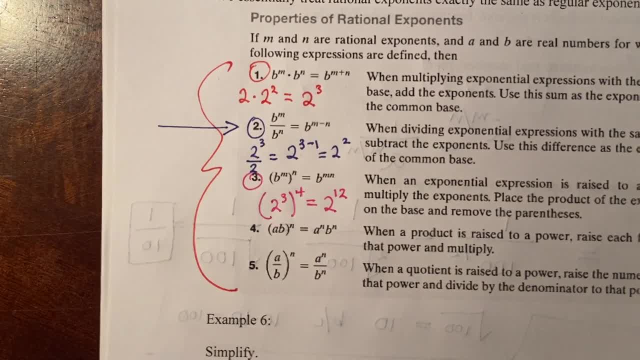 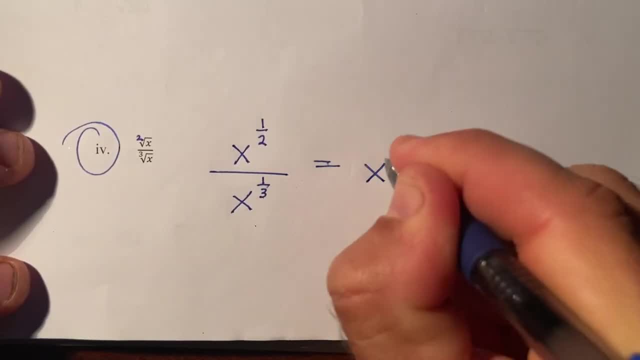 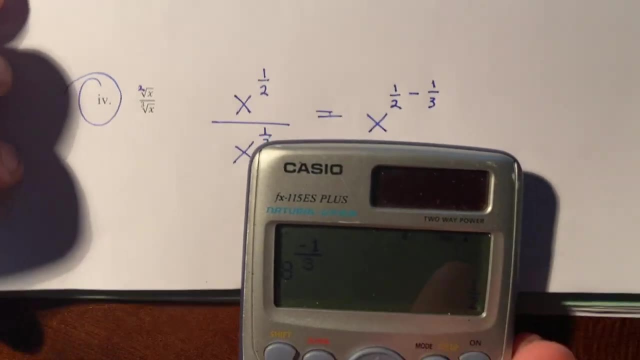 We take the upper minus the lower, So I'll have x to the 1 half minus 1 third. Feel free to use the calculator to help you out on these little intermediate steps. So I'm just trying to figure out what that is. 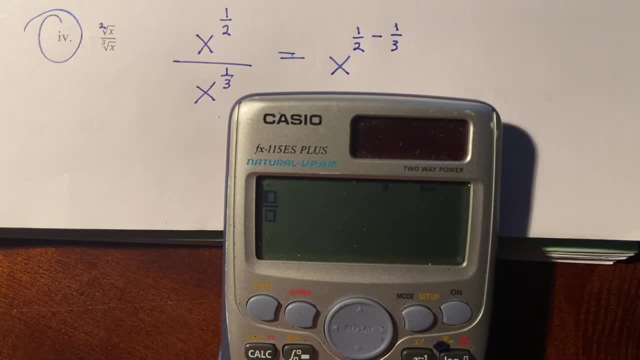 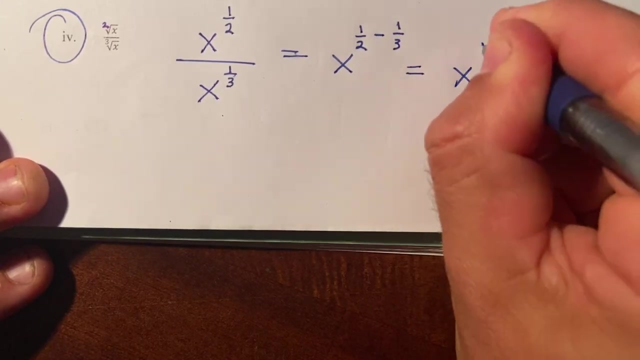 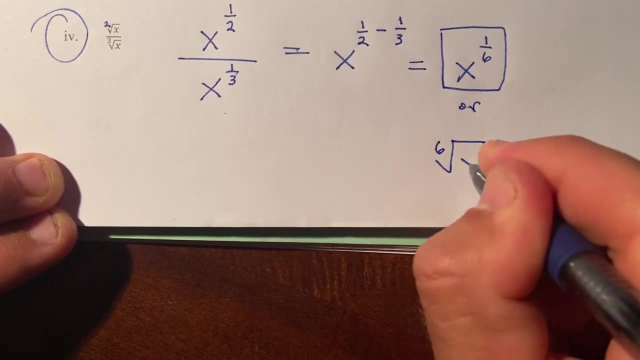 What that resulting power is. So I can go fraction 1 half minus 1 third, It equals, I get a sixth. So you can leave this as x to the 1 sixth, Or you can leave that as the sixth root of x.